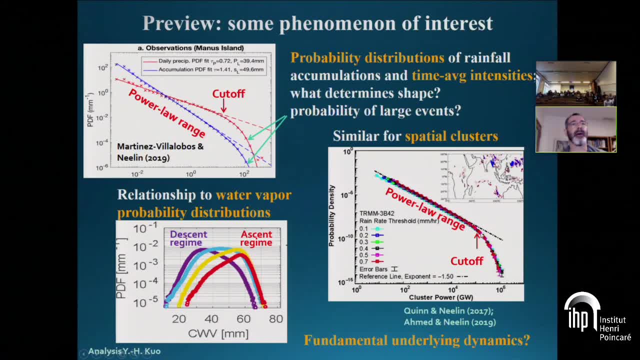 Can we get explanations for this and why this cutoff that separates these two ranges happens where it does, physically speaking, And then when we move to probability distributions of the column water vapor itself, they have characteristic shapes between, say, an ascent regime where you have low-level convergence. 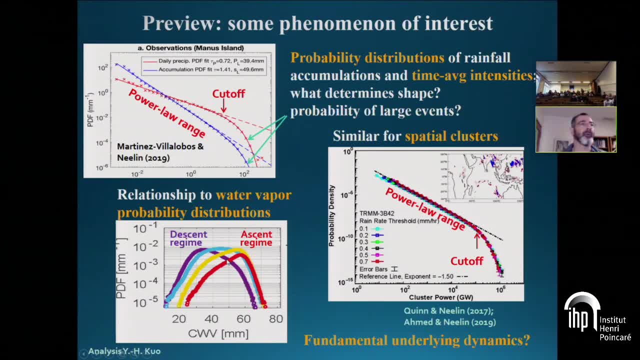 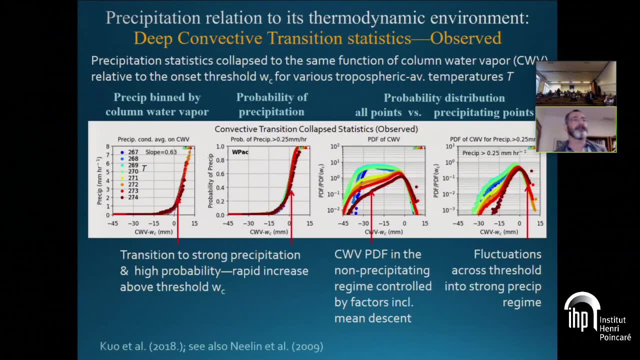 and a descent regime. Can we give you reasons for why you have those shapes? What's the fundamental underlying dynamics? So I'm going to look at first observations and then model statistics in a particular form here. These are a set of four panels that are all related to each other, and I'm going to be 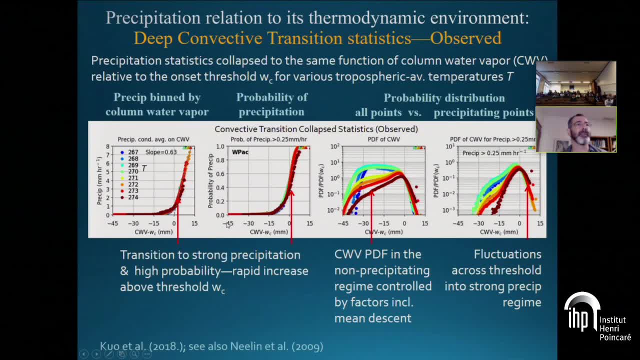 showing you models in comparison to these observations. So let me take a moment to explain what you're seeing. On the leftmost panel you have a conditionally average precipitation. This is the average precipitation as a function of a measure of water vapor, although it's 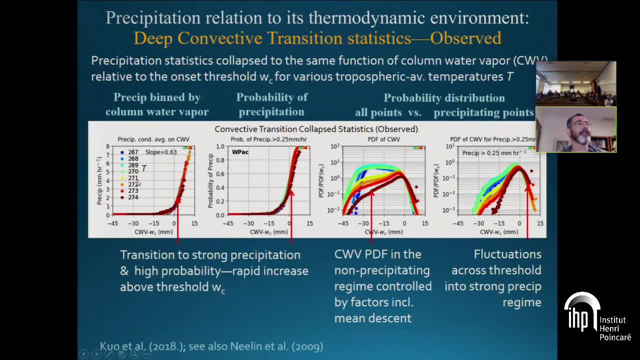 a particular measure that I will have to elaborate on. The different colors are different bulk temperatures. They're a tropospheric temperature measure And the different curves have the precipitation, the conditionally average precipitation, increasing rapidly at a particular value for each temperature. 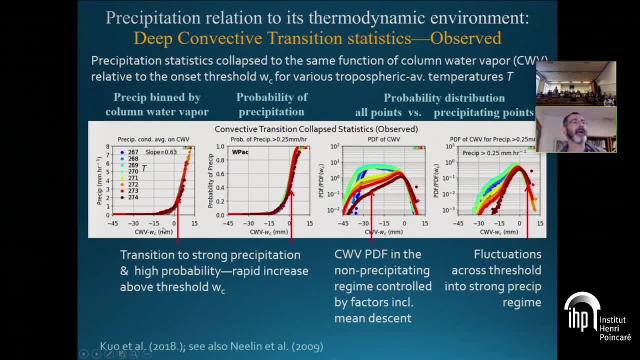 The value I'm characterizing, the sharp increase, has been subtracted so that these curves collapse with one another for each of the temperatures. And this dependence is not simply saturation, It's something more complicated I'll get to in a second. If you do a measure of the probability of precipitation exceeding some modest threshold, 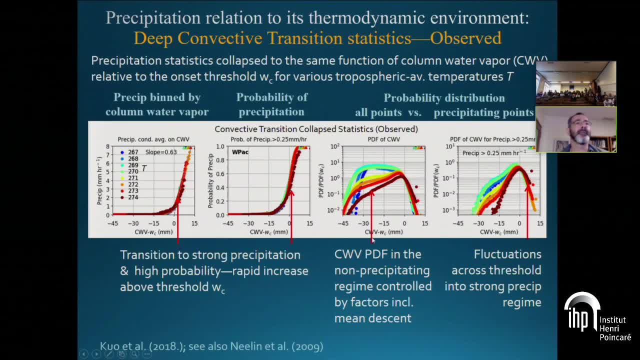 you get a similar rapid increase in collapse. And then, if you look at how the thermodynamic environment itself is in terms of precipitation, you get a similar rapid increase in precipitation. So if you look at the rapid increases in precipitation, the rapid increase in precipitation is just. 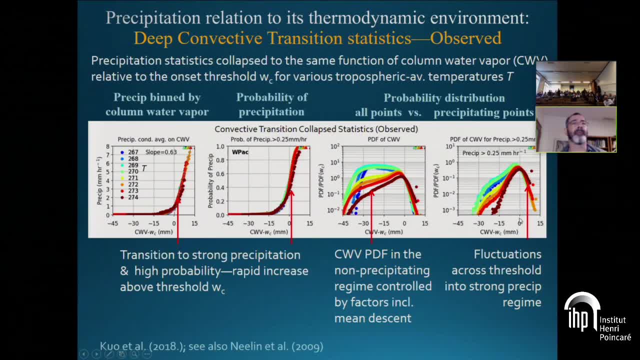 the same as it is in terms of precipitation. But if you look at the precipitating points, you tend to have them clustered around the value where you had that rapid onset. And if you look at the column water vapor relative to its critical value, it does out. 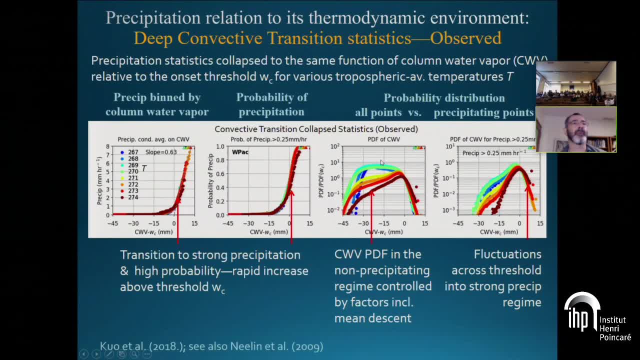 in the non-precipitating regime here, various things that will be governed by other dynamics, And when you get up to the region where you have strong precipitation on setting, you tend to do the same thing over and over again where you have this steep drop. 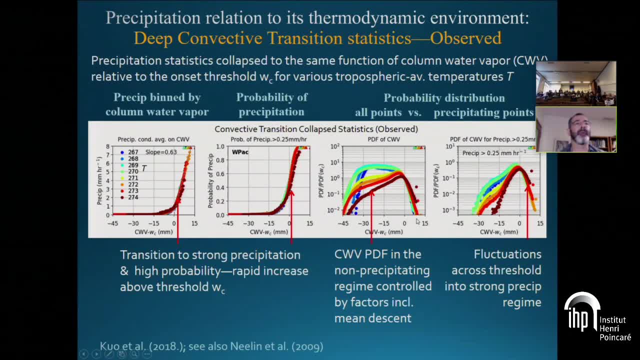 Essentially, you go into this regime, you are raining very hard and dissipating buoyancy, and so you have a drop in the probability of remaining up in that regime, but it has a finite scale over which you tend to hover in that regime. now it is worth taking a moment to put perspective on this. 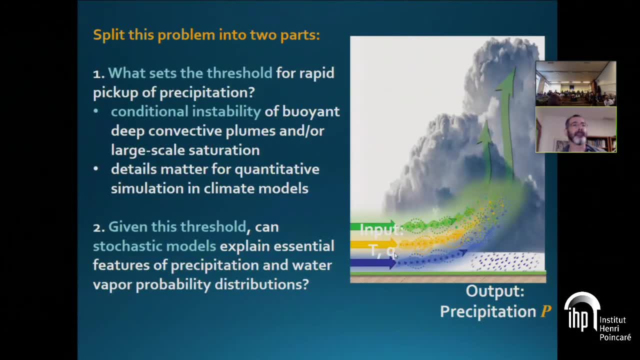 before coming back to the same diagram. so if we think of our convective system, here the inputs are a profile of temperature and moisture and the output we can think of as precipitation. here we're splitting the overall problem into two parts. one is what sets the threshold where you get the rapid onset of precipitation in the tropics. this is primarily 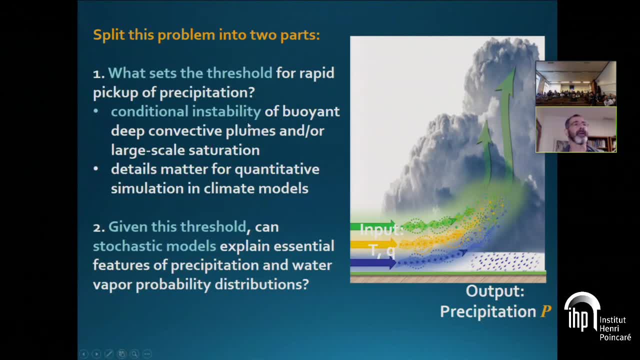 conditional instability, and that's what i'll focus on today. so you get a buoyant, deep, convective plume when your water vapor and temperature reach a certain configuration with respect to each other, and the details of this matter a great deal for the quantitative simulation in 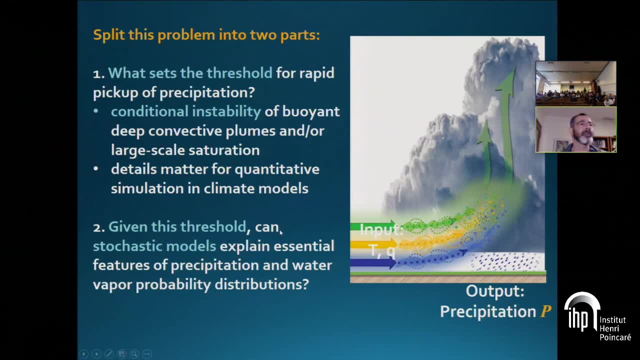 your climate models, as i'll show in a moment, and then most of the talk, the stochastic part, will be. given this threshold type behavior and this rapid increase, can you explain a number of important features about the probability distributions of precipitation? so i'm just going to show you one slide background. brief word on the threshold. 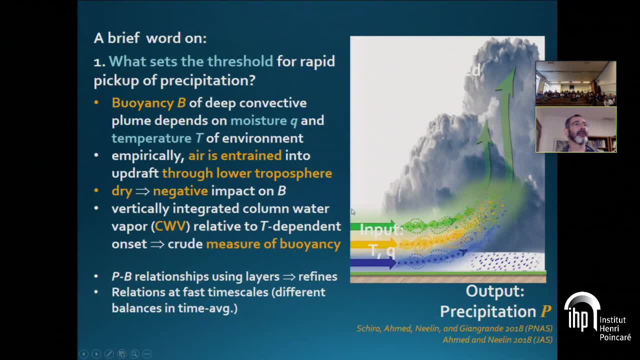 itself. um, so you're going to have some buoyancy of a deep convective plume, depending on these inputs: moisture and temperature. um, empirically, there's evidence that air is being entrained, whether dynamically, in coherent flow, the where the way the mesoscale community likes to draw it, or 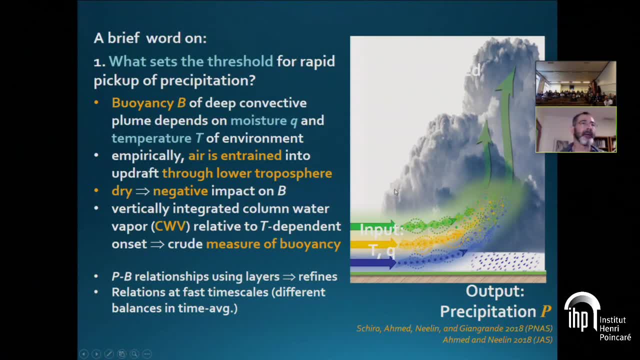 in turbulent, um uh flow the way conventional, um you know, cumulus modeling uh tends to think of it, or more likely some combination of the two. in any case, you, you entrain air through the whole lower troposphere in a manner that gives relatively equally weighting to layers through the bottom. 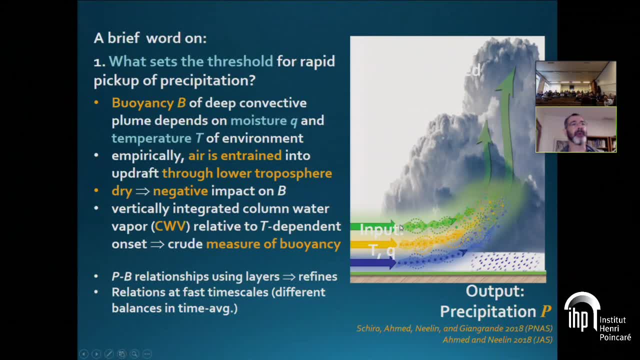 four kilometers. of course, if you're dry and bringing in dry air, you tend to have a negative impact on your convection and between those various factors, of course, if you're too warm, you also have a negative impact, although you're increasing the amount of water vapor, your air can. 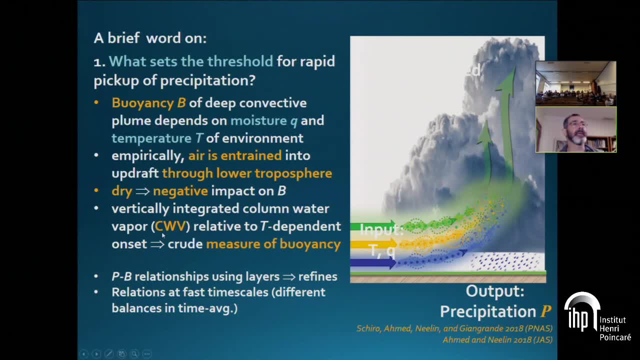 hold between them all. the. the integrated column water vapor, which we have a lot of observations of from satellite, ends up being a sufficient measure of the lower tropospheric water vapor here that that relative to its temperature dependent onset becomes a crude measure of buoyancy. and in work that i can't talk about today, you can refine this, these measures of buoyancy, using 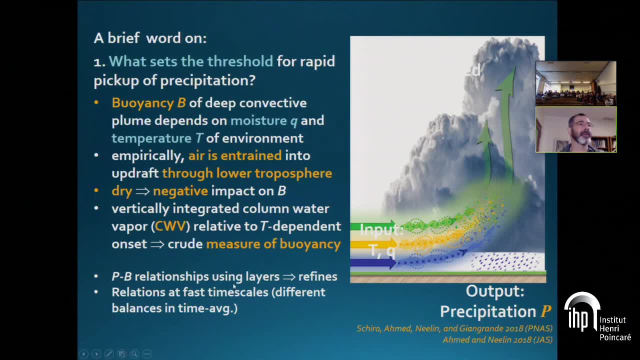 different layers, and that's a that's a subject of a talk all by itself. then i should also remember to mention that these, um, everything i'm saying here holds for relationships fast time scales. you're looking at instantaneous to hourly type beta in all of this talk and, uh, because the the 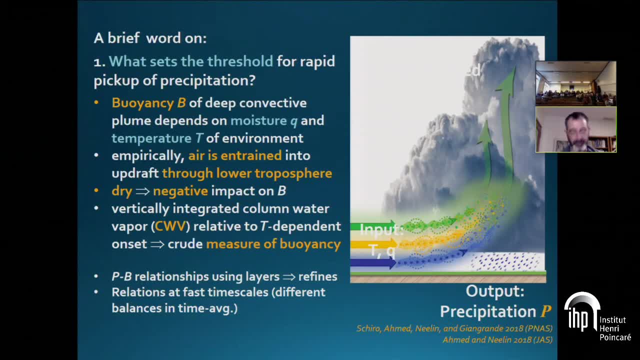 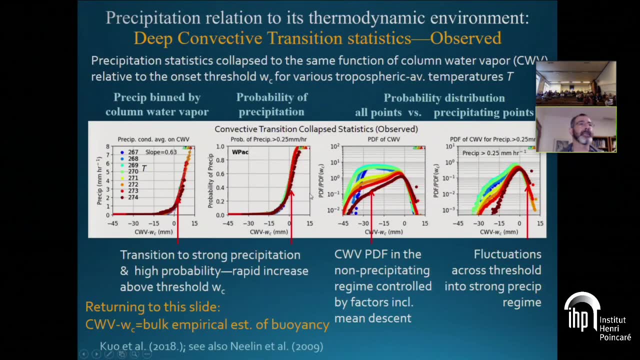 long-term time average obeys different balances involving different large-scale balances of the energy and moisture equations. okay, so back to the exact same uh slide that i was showing earlier, and what we've added by this little uh sidestep is that we are interpreting this column water vapor. 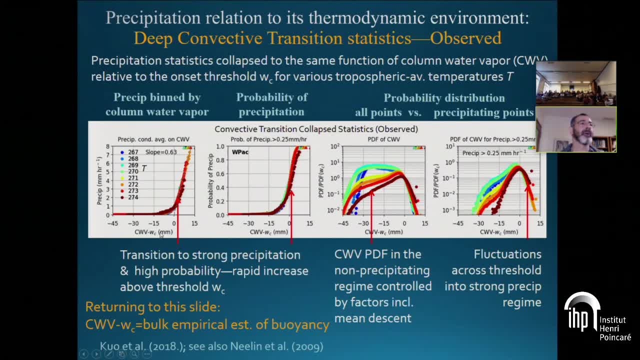 relative to the temperature dependent value where it onsets, as an empirical estimate of buoyancy. and so in the stochastic model we can run a column water vapor equation and use the fact that we have this rapid onset of precipitation um as an empirical input, uh, establishing what happens. 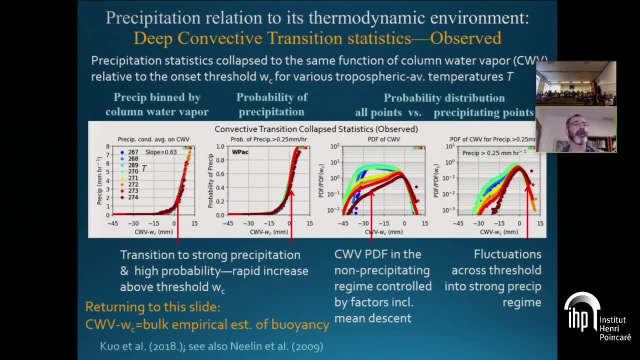 when we hit the precipitating regime. okay, so these are the observations for the. you know the onset and precipitation, how long you spend, uh, in the non-precipitating versus the precipitating regime, and what part of that is for precipitating points. let's look at some models to see how. 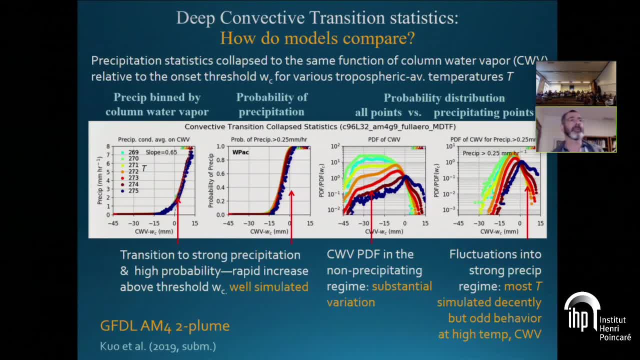 well, they reproduce this. so here, for example, is the gfdl model, same format of diagram. uh, this is for one particular convective parameterization and it's doing pretty well. the onset is well represented in conditional average and probability of precipitation. your precipitating points are fairly well confined near this onset. you have some interesting. 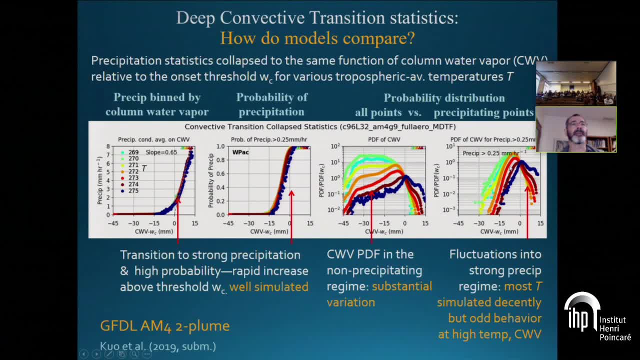 behavior as you move. remember these different colors are different bulk temperatures of the troposphere. as you move to the warmest temperatures, you're getting some odd things, including this temperature, and then you have this extra bump at very high water vapor, going on the model that we 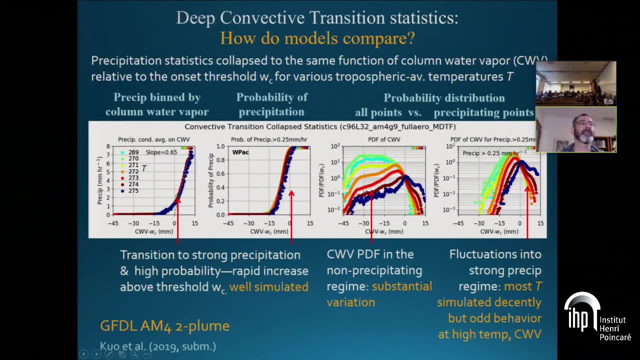 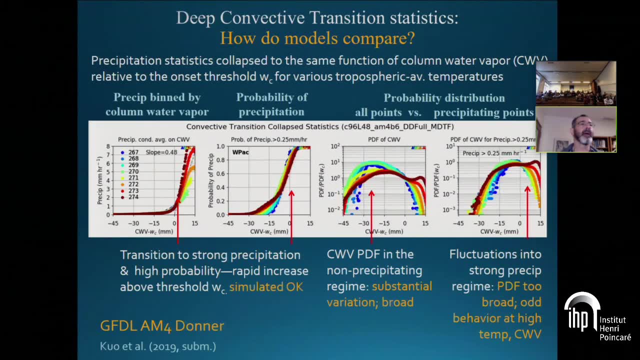 did not see in the observations. and then you have this spread out in the non-precipitating regime. that will be something to explain later. if we switch convective schemes in the same model to the donner scheme, you get qualitatively similar features, but the details change quite a bit. your. 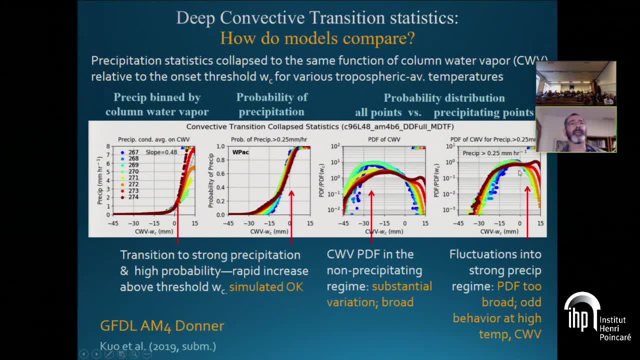 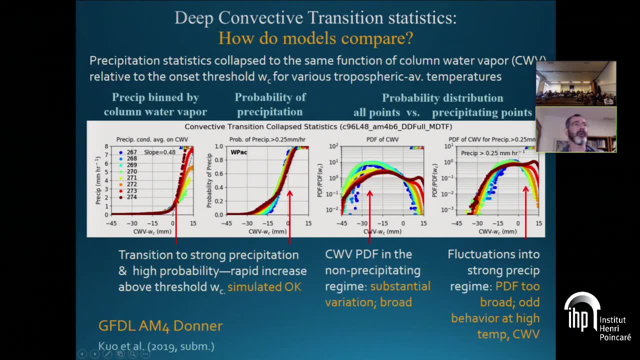 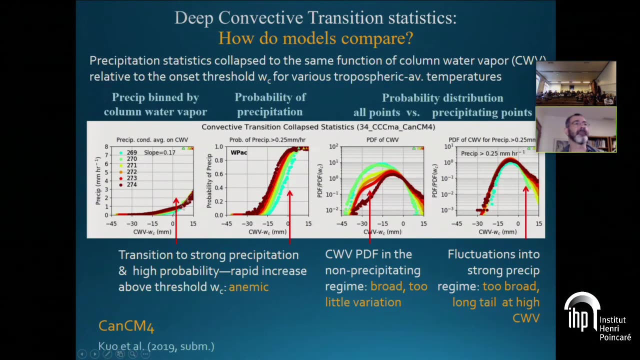 onset is now a function of temperature and you have a very broad distribution here. still this sort of effect at the very warmest temperatures. and just surveying a couple more models, here's the canadian model particular version. it has some version of the pickup but it's a little. 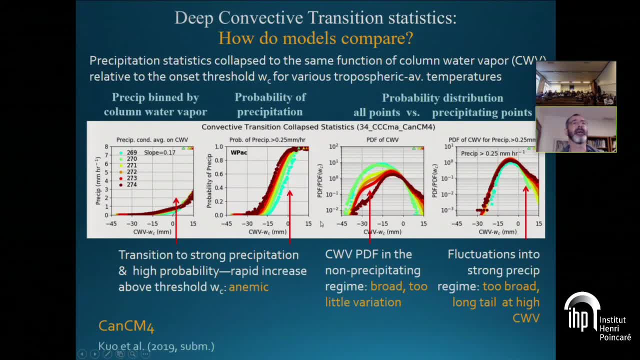 bit anemic and it sort of has a two-stage effect. so, pointing to questions about the convective parameterization and the large-scale parameterization and very broad precipitating pdfs, if we look at ec earth it's doing basically great. the pickup perhaps doesn't extend as 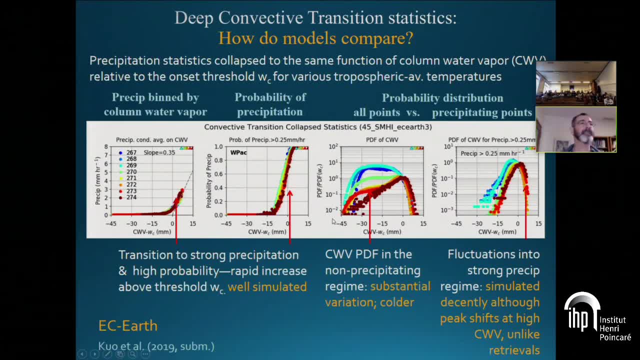 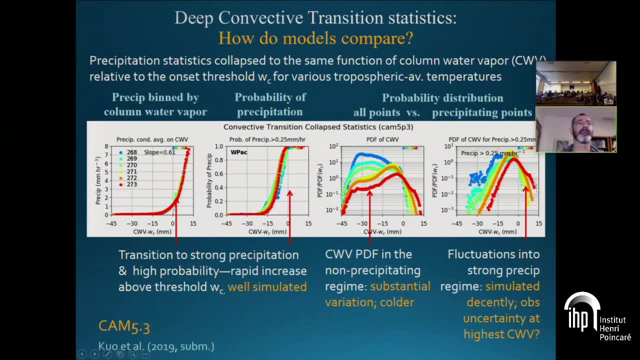 high as in observations, but everything is more or less in the right place. if we look at cam 5.3, it's also doing quite well. you have this tendency to different behavior, this little extra bump at high, very high temperatures, and i should point out that if you're going to 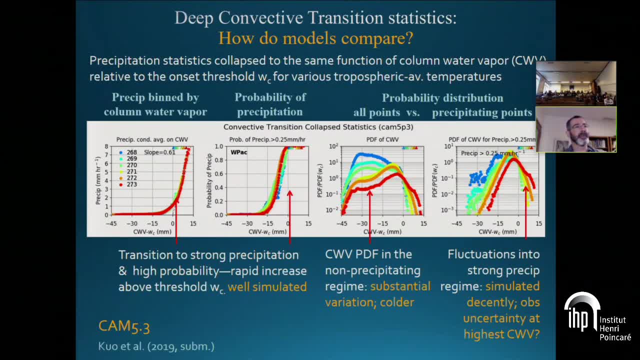 use these models for global warming. the fact that you're doing things a little oddly in the high temperature, high water vapor regime is something that would be of concern. we can just briefly check what if you switch to a super parametrized version of the same end car model. 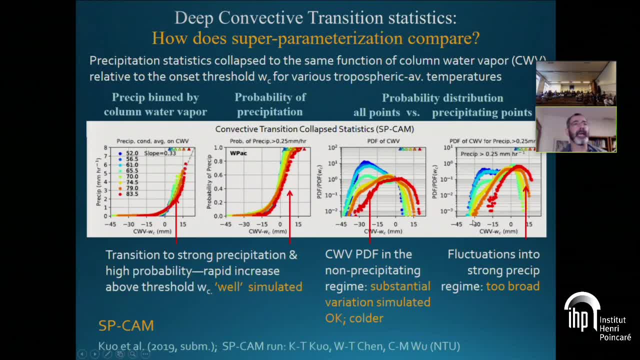 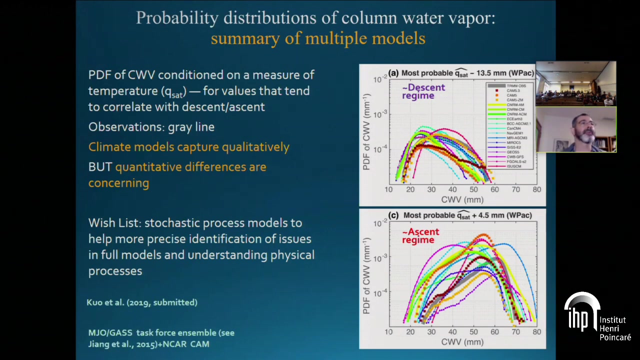 in other words, you're running a cloud resolving model under every grid of a grid cell of the climate model and again you've got qualitatively the correct behavior, the pickup. but you tend to have rather broad pdfs for this model. so the precipitating points. so it was not a magic bullet in and of itself to use the super. 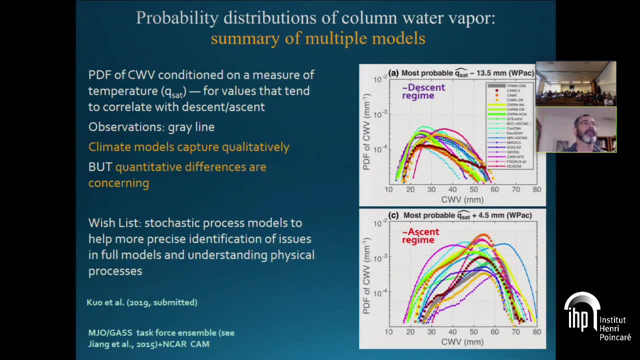 parameterization. okay, so summarizing that, just putting multiple models, the ones you've seen plus other ones. this is for the- you know probably the distribution of column water vapor shown here, for something like a descent regime and an ascent regime. the models are doing generally the same. 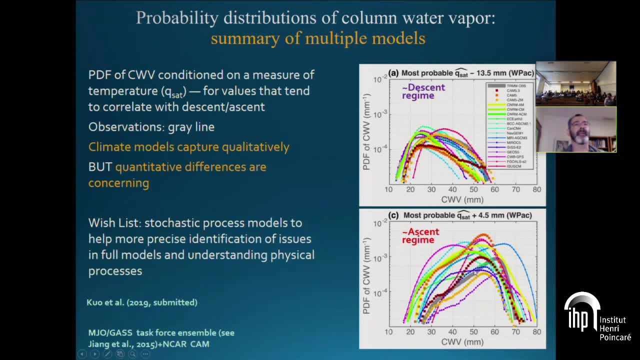 thing: peak at low water vapor here, drop at low water vapor here. drop at low water vapor here, drop dropping off ascent regime packed up towards the place where the onset would happen, but with a fair amount of variability in exactly what goes on there. so you'd like to have process models in. 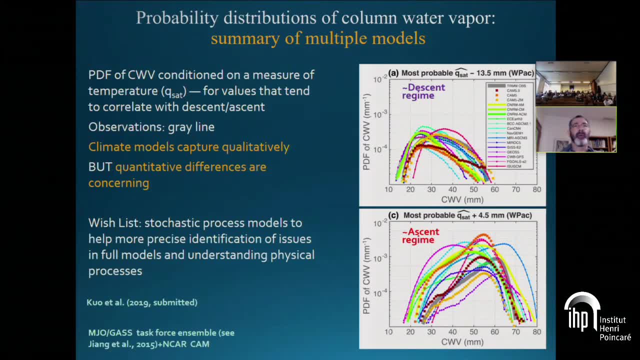 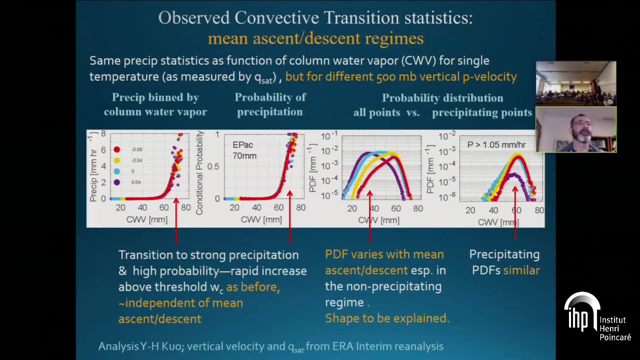 this case stochastic models, to help identify what is the physics underlying this, both in observations and the type of sensitivity that you might get in these full models. one more thing, in this same format, which is showing the statistics you just saw, but broken out by mean, ascent or descent regime, using 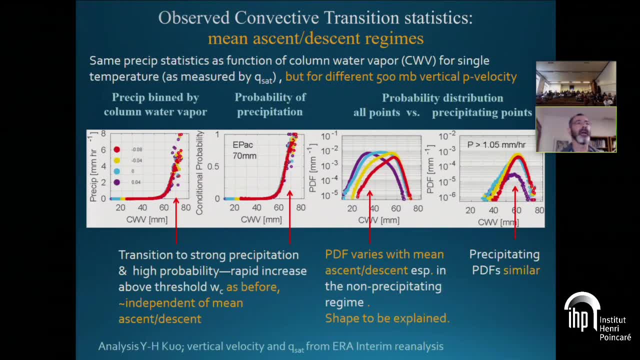 monthly average 500 millibar vertical velocity from the era interim reanalysis. this is in observations. the pickup in the conditional average precipitation probability. precipitation is going on same as before. this is shown for one particular temperature and the different colors are now calcified. so the last 그метport to flat bottom. você sabe essa primeira. 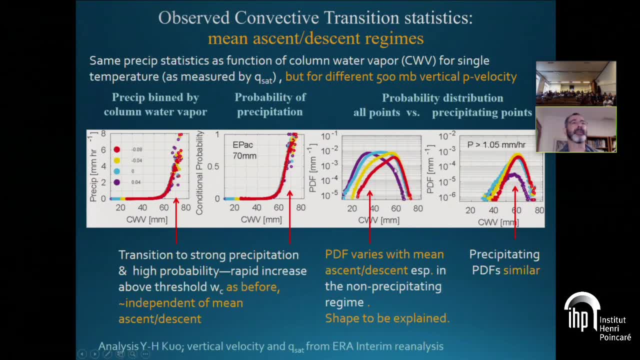 é essa parte aqui, passage que posiciona set de dengan athenas um. Whereas if you're in the ascent regime- low-level moisture convergence- you tend to be more commonly confined towards the onset of precipitation, You spend less time in the dry regime out here. 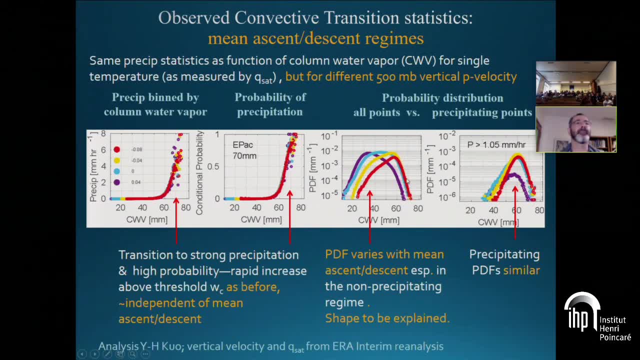 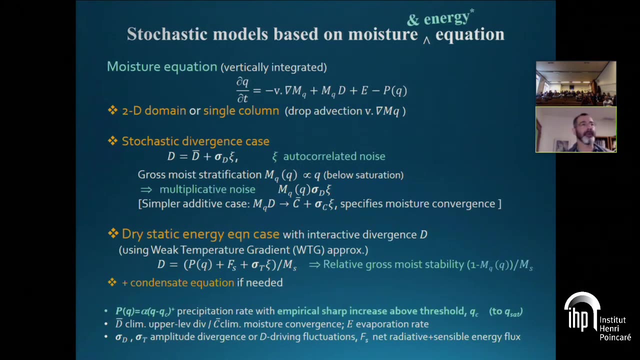 But once you're in the precipitating regime, you tend to have a drop in a similar way in each case, with the large-scale dynamics being less important. Okay, so the stochastic model to explain this behavior, plus some other things involving the clusters and the probability distribution of precipitation itself. 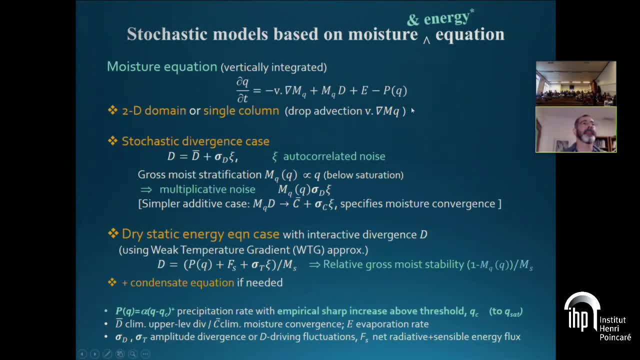 At the top is a moisture equation. You have the time derivative of moisture and then you have a moisture convergence term. here This MQ is a vertically integrated moisture. Our Q is the column water vapor And MQ is proportional to moisture, but it's containing a factor that involves the vertical structure of the wind and the moisture relative to each other. 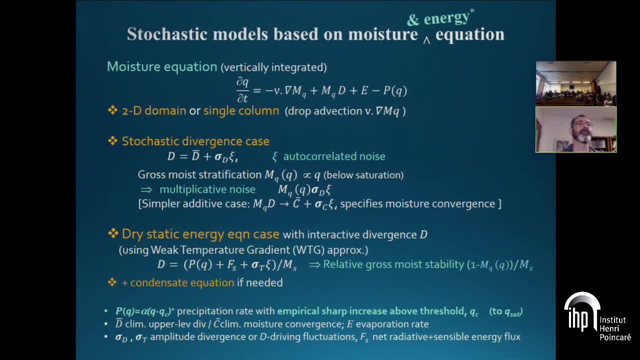 If it was just a layer model, this would just be the moisture itself. You're evaporating and then you're precipitating, And the precipitation is a function of moisture that captures that empirical sharp increase. Here we're just using a wrap function in most cases that I'll show. 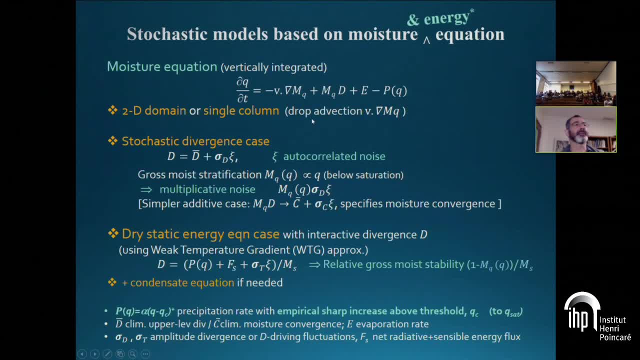 You can. so you've got this moisture budget. You can run this in a 2D domain, or you can look at a single column at a time, and I'll show you examples of both. What do you do about the divergence? 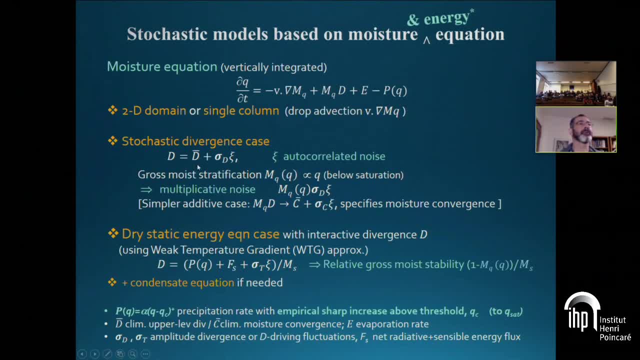 The simplest case is you specify it as a climatological divergence plus an autocorrelated noise. Note that it'll be a multiplicative noise because this is essentially proportional to moisture until you saturate, and you can, for simplicity, also switch this model out with with one where you replace this whole moisture convergence term with just a mean moisture. 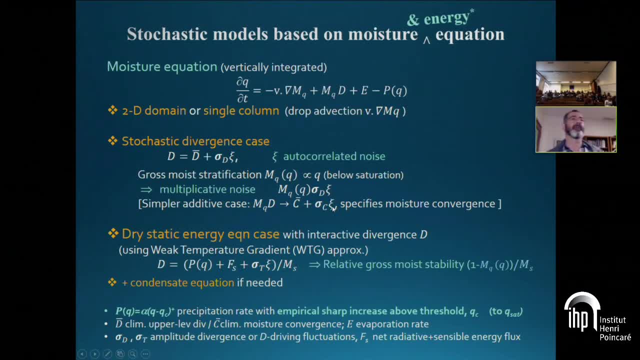 convergence plus a specified noise that's for. that will give you some results that are relatively similar for understanding, for instance, pdf precipitation. now there's going to be an important feedback when you're raining from the temperature equation, or dry static energy equation vertically integrated as we're using here. more specifically, your divergence is going to be. 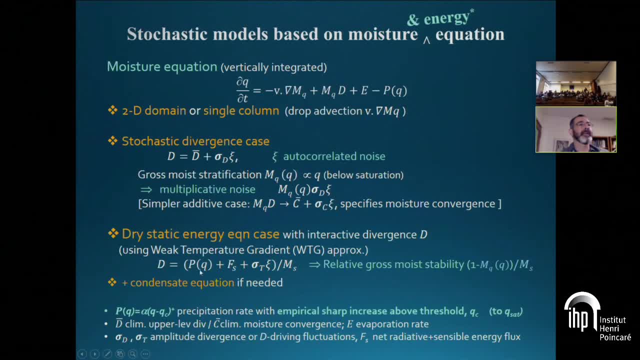 balanced. the adiabatic cooling is going to be balanced by the latent heating, which is proportional to the precipitation in the vertical integral, and so you're going to be able to do that. you're going to get a feedback. you're going to have a net flux into the column, tending to force. 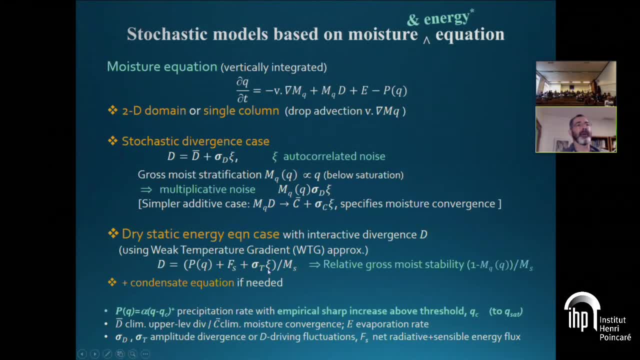 this. you're going to have a noise term from all the gravity waves and so on, changing your d by dt term. that has been as well as v, dot, grad t and any random fluctuations in the flux wrapped into this sort of divergence driving term. so your divergence will have a feedback. 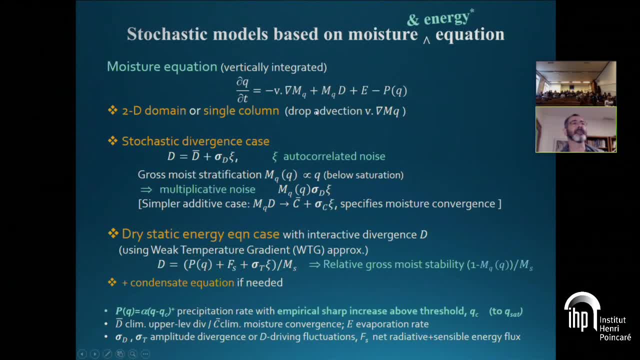 with the precipitation and if you check about substituting this back into this equation, you'll see the precipitation arises twice and it's going to end up multiplied by a term. there's a parenthesis slightly wrong here, but a term which involves the moisture stratification term relative to the dry stratification term, ms. so that'll be a relative gross moist stability. 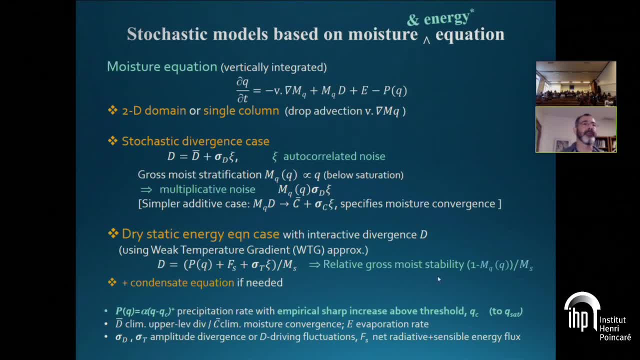 measuring the amount of net energy you get when you cancel the diabetic heating and the adiabatic cooling for a large amount of time. so that's a little bit more complicated, but it's going to be a large scale, uh, upland. okay, so that's our um, our simple thermodynamic stochastic model that we can. 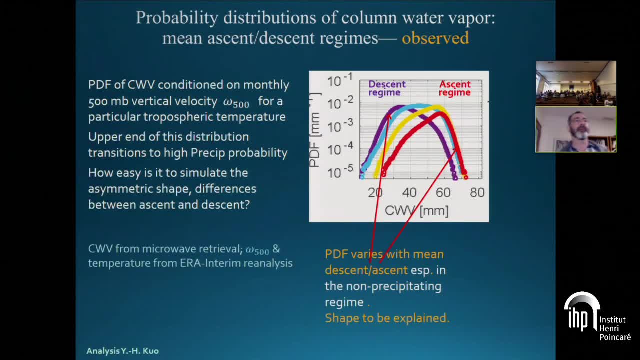 use to you to try and explain some of these features now let me remind you- i'm just going to zoom in on one panel of the thing that you saw last time. this is the pdf of moisture when you're dividing by ascent regime and descent regime in the descent regime, and observations. 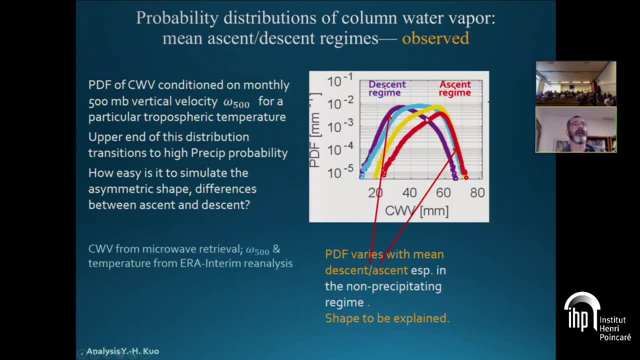 you spend a long time at relatively low water vapor, but you slowly drop until you hit in probability, until you still sometimes hit the precipitating regime, and then, if you're in an ascent regime, you spend more time up there. can we explain the shapes of these distributions from that stochastic model? so here's what you get. 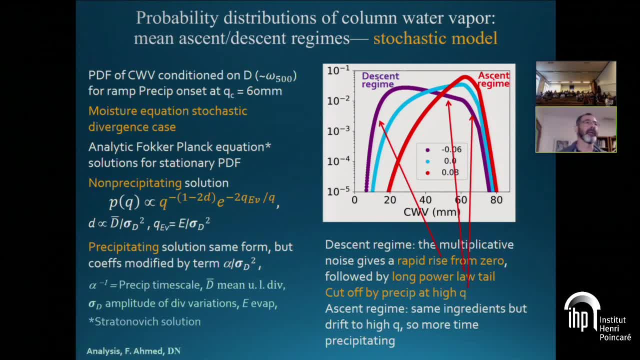 these are actually analytic solutions from a version of that stochastic model you just saw, including the multiplicative noise, your uh forming the fokker plank equation for the stationary distribution. solving that analytically. and the elements that you get in the non-precipitating regime include a typical scale. 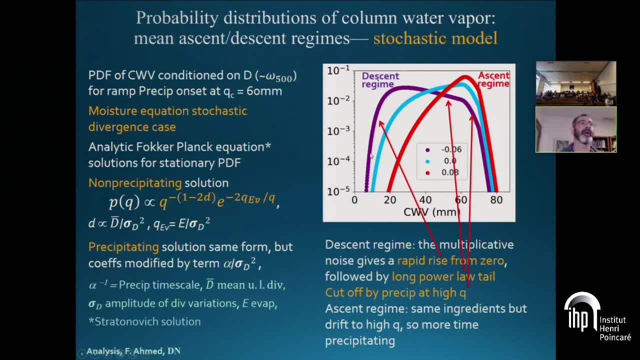 with a 1 over q. that's giving you your rapid rise from low moisture that you see here, and that scale involves the evaporation relative to the amplitude of the noise. and then you get this long power law regime, that whose exponent depends on the divergence. so in the descent regime, even though you 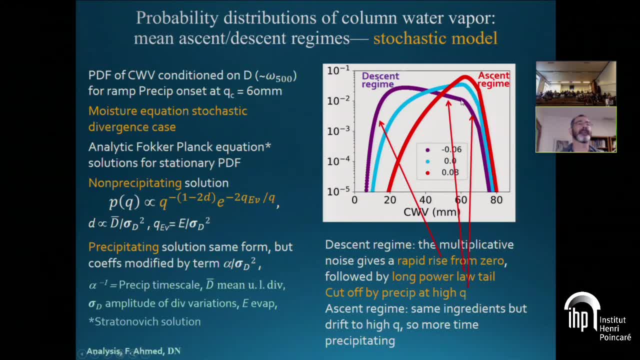 have a peak at low water vapor. your noise will sometimes manage. you get to get you up to quite high water vapors where your precipitation and then you enter a new regime. um, the precipitating solution is somewhat more complicated, has generally the same form, but the coefficients get modified by the fast time scale. 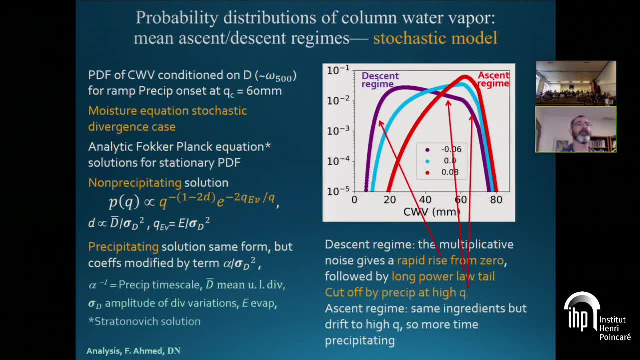 of the precipitation in that empirical rapid onset, and so you get a rapid drop of the probability of precipitation with a characteristic scale that depends on that, that time scale in the precipitation. and that goes on approximately the same, whether in the ascent regime, the low level convergent. 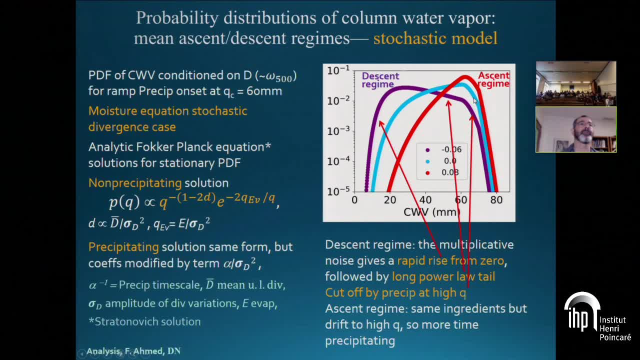 regime, or the low level divergence regime here, or neutral in between, and then once in a while, you'll manage to hit large scale saturation. essentially, you'll have reached such high water vapor that you saturate your column, in which case we've parametrized that as a steeper. 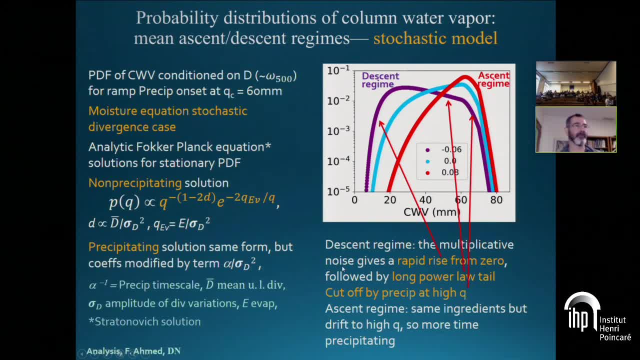 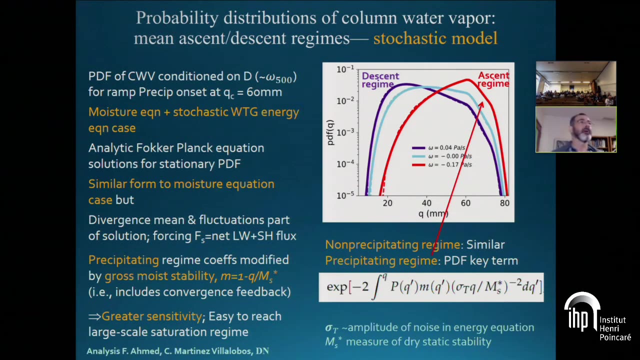 drop down here a faster time scale of conversion of water vapor. so that's using the moisture equation only with the specified divergence case. if we move to the one that also has an energy equation and includes the moisture feedback, we get a very similar form. it's just a little step more complicated than what we saw before, so i'm not giving you the 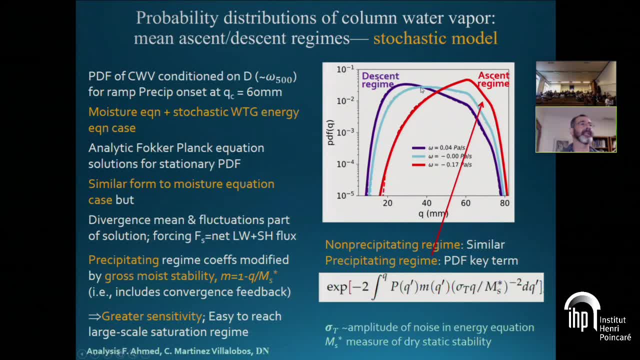 whole expression. the descent regime is an exact analog, except it's forced directly by the flux into the column, and so you get for the descent regime spending a lot of time at low water vapor. but this long power law tail up to the onset of precipitation, and then this steeper drop. 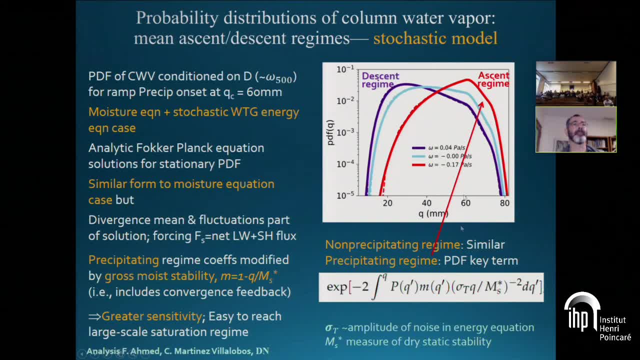 but the coefficients in here. the dependence in here has a more complex form. a key term involves an integral of the precipitation as a function of moisture, which is the loss term, this gross moist stability, which has a one minus moisture relative to some dry stability term here, and that's reducing the effects of this loss by 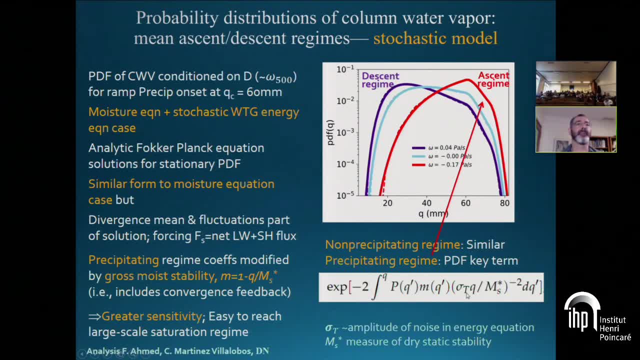 additional moisture convergence and it's all relative to measures of what's happening in the, in the variance of the of the noise, so there's greater sensitivity here. you can change this shape. in fact, if you have a region of negative gross moist stability, then this curvature can change and you can actually get a little bump before the saturation. 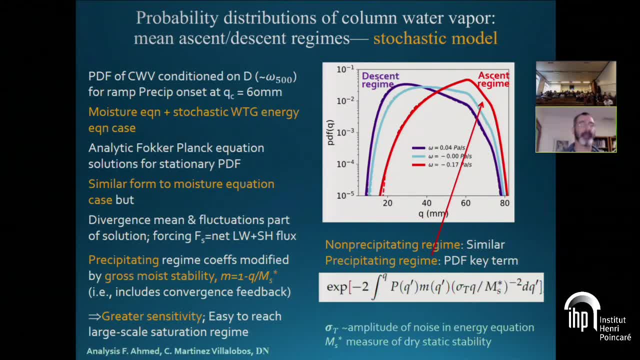 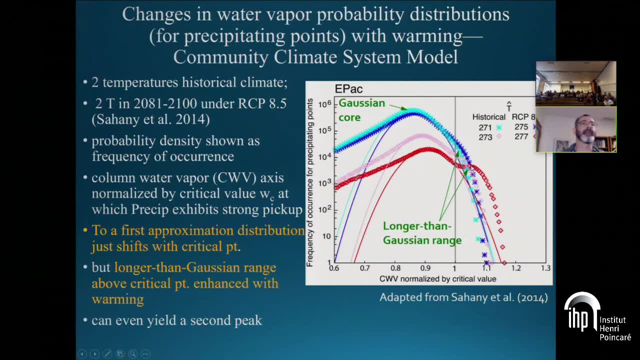 regime. so it's much easier, it can be much easier to reach the large scale saturation regime. so remember, in the models in current climate we have these funny double bumps, sometimes at high temperature. this is a different example of a pdf of water vapor relative to its critical value. it's. 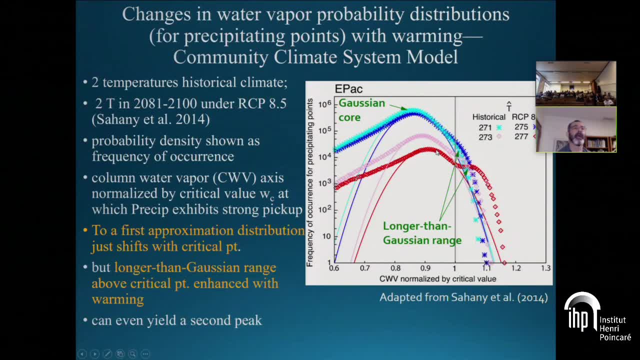 a slightly different measure of the critical value for two cases. one is a historical run and one is a representative concentration pathway. 8.5 global warming run. you're showing two temperatures for each case- a lower temperature and a high temperature, and as we move from the 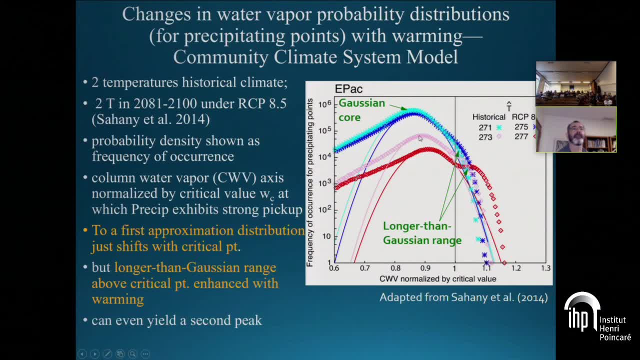 move from, say for the higher temperature case, from the current climate to the future climate. everything stays more or less the same in the bulk of this distribution once it's moved relative to its critical value. but the longer than gaussian range out here changes quite a bit, so you're. 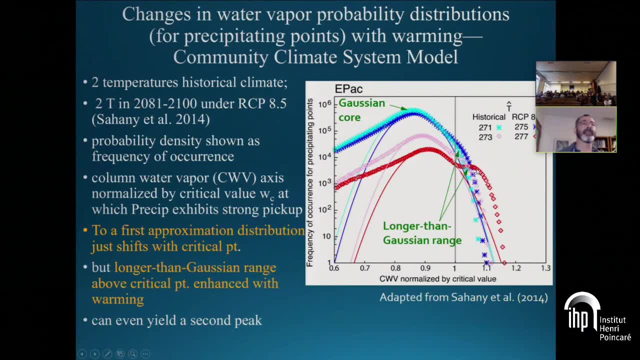 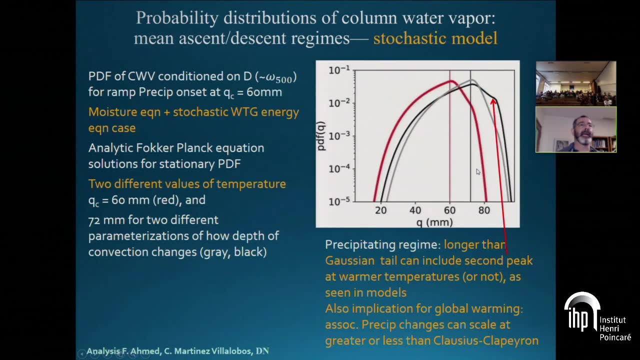 spending more time in these extreme event ranges. can we get an analog for that in the um simple stochastic model? well, yes, this is uh, showing in red here a representation of the current climate where you have a certain value for the critical water vapor for onset and then 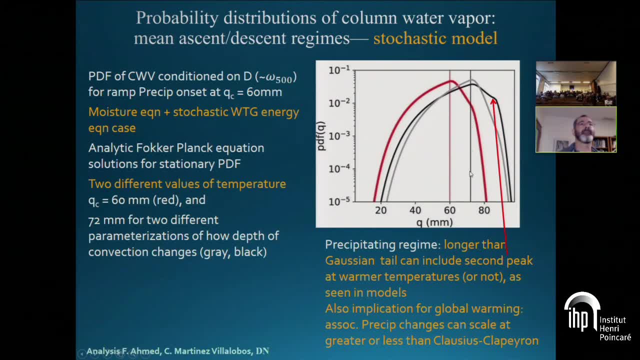 another case at a warmer temperature, representing the future climate where your onset is at a higher value. there are two curves shown here and they make slightly different assumptions for what happens to the drip of the dry stability as the climate warms relative to the change in the onset for convection. 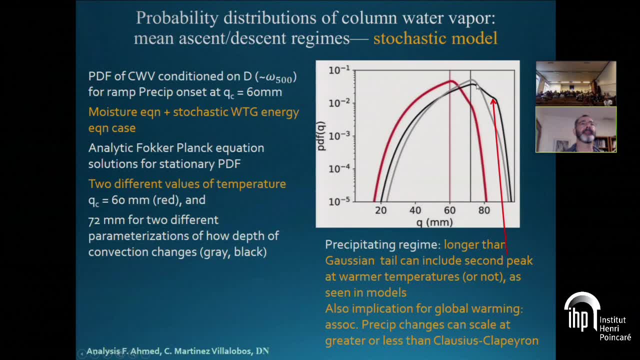 in one case you continue to get a fairly steep drop in the probability of your extreme event- uh, extreme water vapor events associated with very high precipitation- and the other case you've begun to develop a bit of a double bump here where you have slightly less adjustment of the dry static. 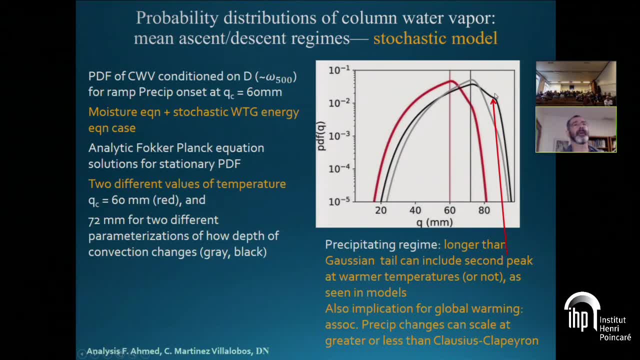 stability and, of course, if you um push this behavior even farther, you can get a full double bump. so this is an analog for what's happening as a function of temperature in the models of current climate and also for what is being represented in the models in a. 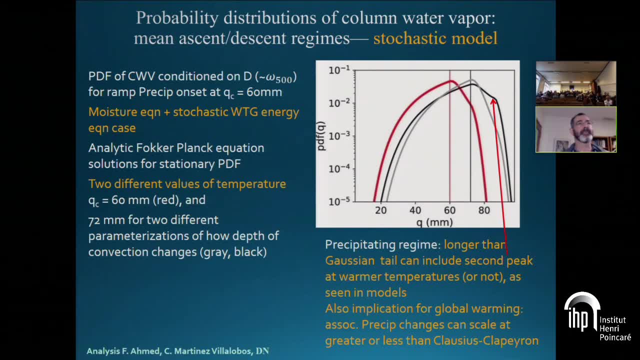 future climate and it focuses you on the particular physics that's relevant to these changes in the probability distribution, the pdf in the um and the high temperature, high water vapor regime. and when you look at the precipitation distributions from such a model, they can scale it greater or less than the closest clipperon depending on what's going on in this. 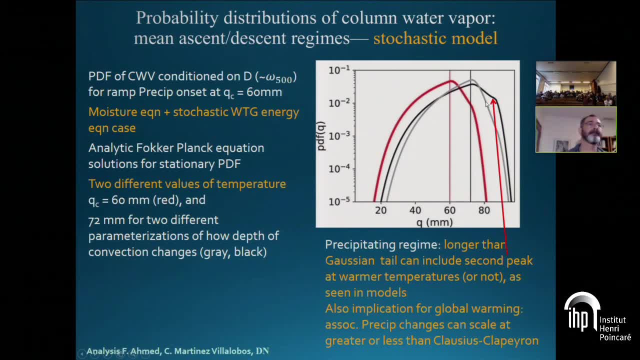 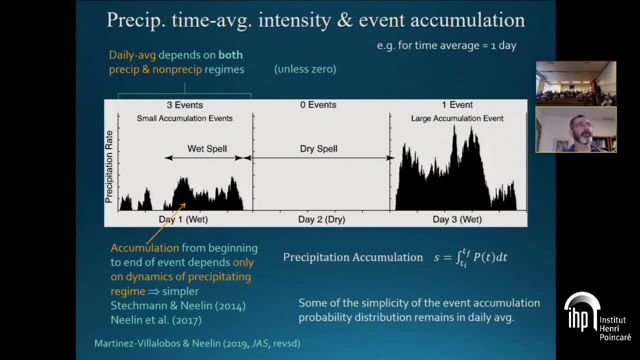 region up here. so it depends on the gross moist stability. okay, so speaking of that, let's move to understanding the probability distributions of precipitation itself. let's begin with a idealized time series of precipitation with the time axis running along here, and in a single day you could have multiple events where the precipitation starts, stops for a while, starts. 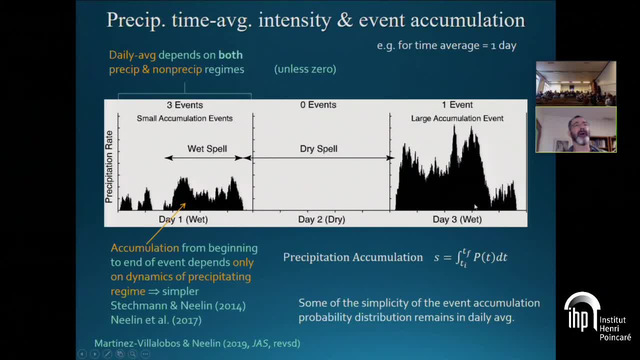 again, stops for a while, starts again, you can have very long events that continue for most of the day. they can even, of course, go over the boundaries of your day. you can have days that have no precipitation. but one of the points here is that if you look at one measure, which is the accumulation of 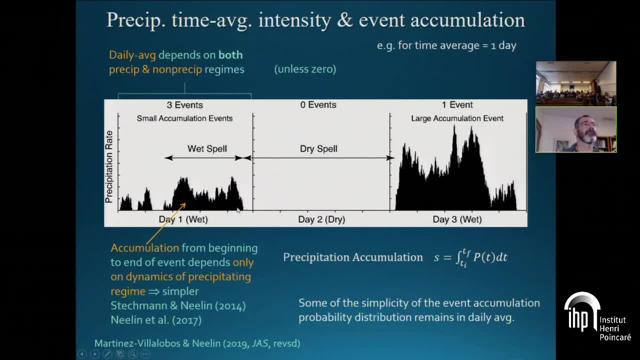 precipitation from when your event started, integrate all the way through until when it stopped. that's actually going to be a simpler measure of precipitation amount in the following sense: it only depends on the dynamics of the precipitating regime. if you look at a daily average or a 12-hour average or a five-day average, you're going to be mixing properties from the non-precipitating 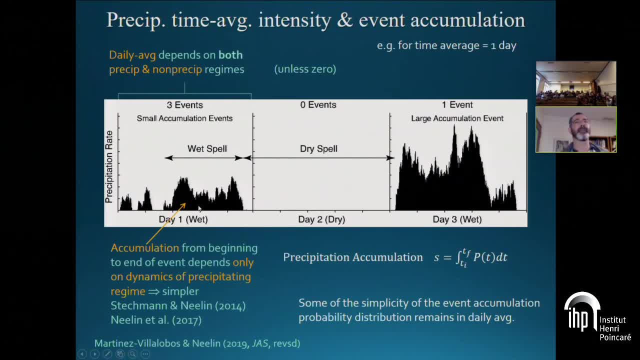 regime and from the precipitating regime, and so you're going to get a mix of dynamical regimes in this that time averaged intensity, and so what we're going to argue here is that, even in the time averages, some of the simplicity of the distribution of event accumulations, which 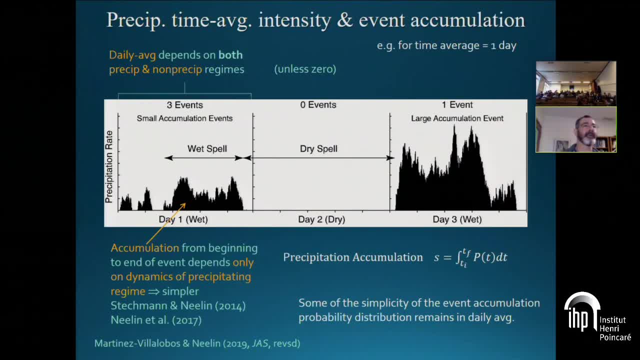 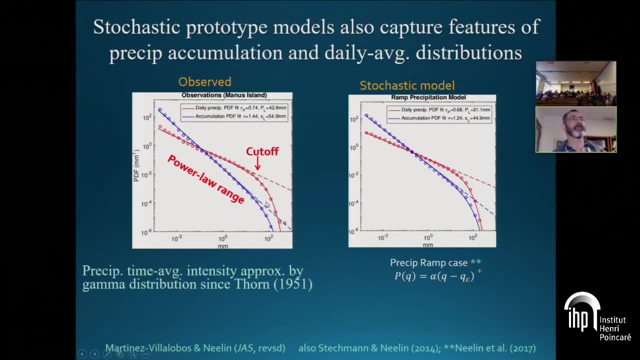 we will also explain- gets inherited by the time averages. okay, so on the left is the observed- i showed this in the intro in the second slide- distributions on a log. log plot of the probability of getting different sizes of precipitation events. the blue line with the steep drop in the power law range. here is the distribution of the accumulation, so rainfall. 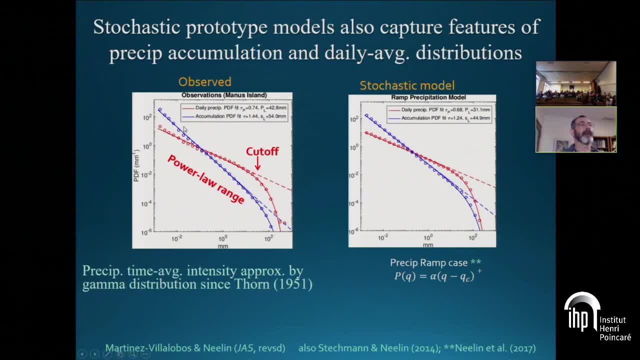 integrated from when an event started to when it stopped and that's dropping at a steeper than neg with a steeper than negative one exponent. in this case it's about negative 1.4. these are for department of energy observation and these are for the different types of perception that we're going to look at. 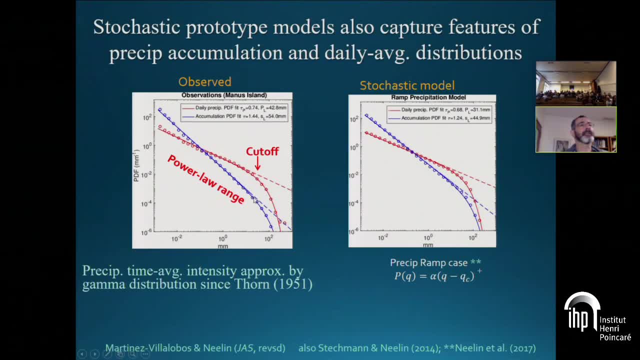 so you can see that this is the field of that graph, we can see that it's our anyway, but we can't measure it. we do it, but i'm going to do it, and so we can see that this is the回 disciplined rate of occurring in different. 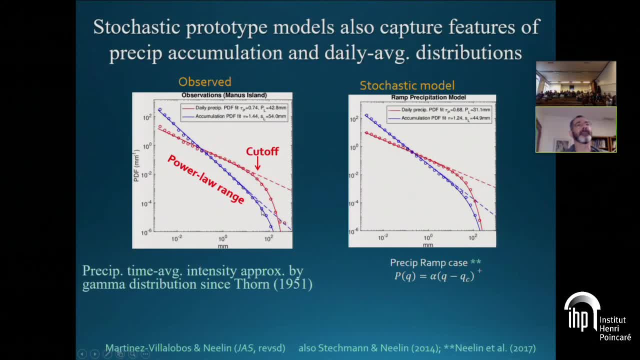 locations at mannus island. you can do it in various places. when you average this up to a daily, you still have something that's- uh, approximately a power law range here. and when you look at this steep cutoff where you begin to drop roughly exponentially- that cutoff tends to match between the averaged intensity and the distribution of the accumulations- then if you look in that stochastic model that i showed you very briefly, then we look at the number of populationbeds. 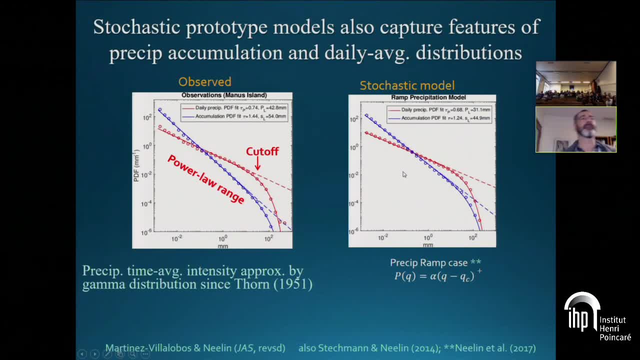 accumulations, Then if you look in that stochastic model that I showed earlier, you can reproduce this behavior rather well. Now, one thing to be said is that the precipitation time average intensity has been approximated by a gamma distribution for decades, starting with Thorne. 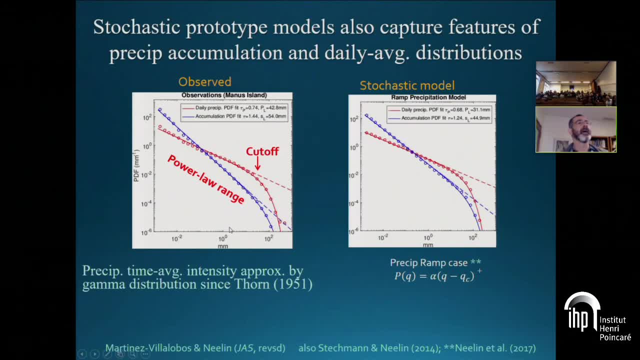 1951 was the earliest I could find, And so, as soon as this exponent is less than minus one, you can use gamma distribution, which will have the power law range in the cutoff, And what we're going to say is that that actually has physics to it, although in the time average it's only 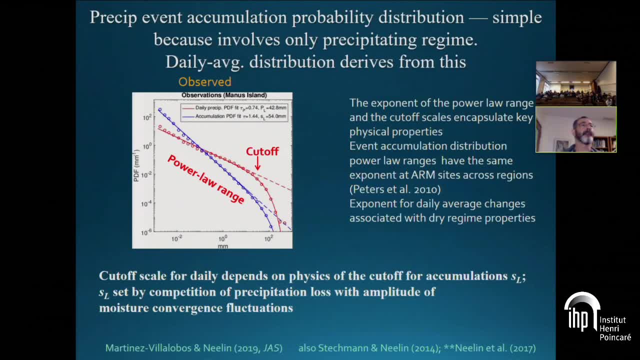 an approximation. Okay, So to summarize, let's talk about the relationship between the daily average and the power law range, And I don't have time to go into the details of this, but simply summarizing the bottom line, Given that you have this accumulation distribution and the accumulation distribution, 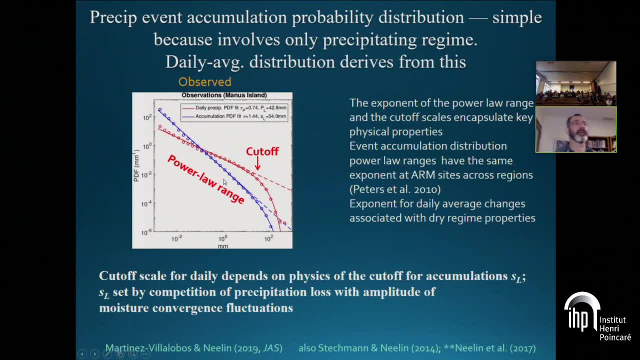 its power law exponent tends to be the same across different meteorological regimes. When you move to a daily average, you're going to be in a given day, often averaging several events, So the amount that falls in a day versus during an event will move probability from the small events to the 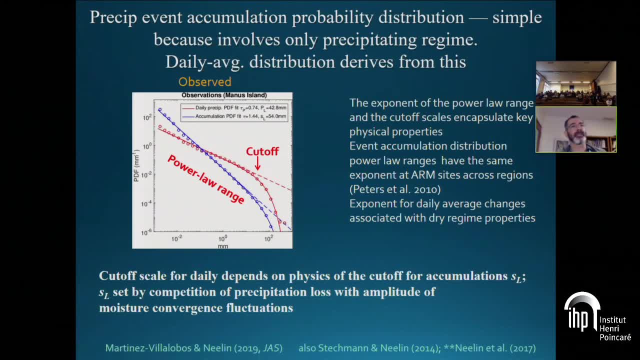 large events. But you're going to essentially be having a daily average which is going to be a weighted sum of variables pulled from this distribution, And you're going to end up with something that, if the time average does not introduce any scale in your distribution, will. 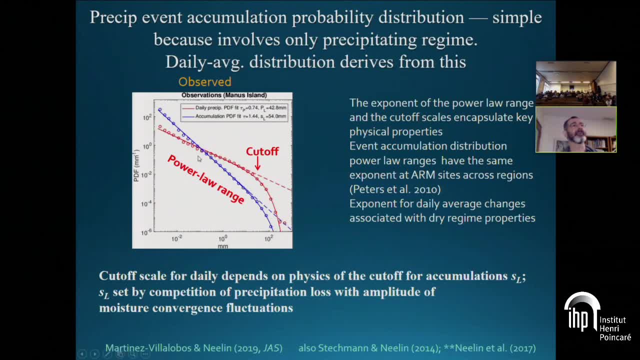 have to be still approximately a power law And it is approximate, not an exact power law here. But you won't have a strong scale dependence here And it'll be a less steep slope simply because you've added up events Once you get to the power law less than negative one. this is similar to saying that if you take 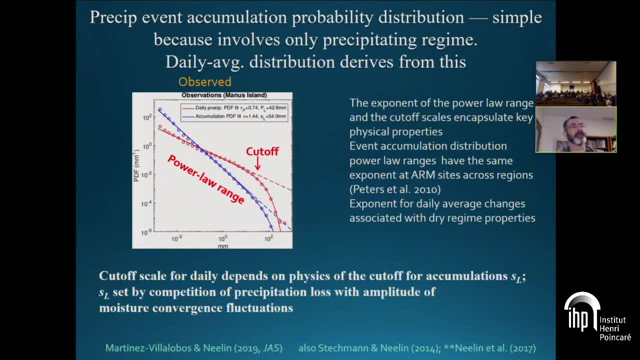 samples from a gamma distribution and you add them together, you will get a variable from another gamma distribution with a less steep slope. So the cutoff scale then is getting inherited from the one in the accumulation distribution. So we'll give it some physics of that. 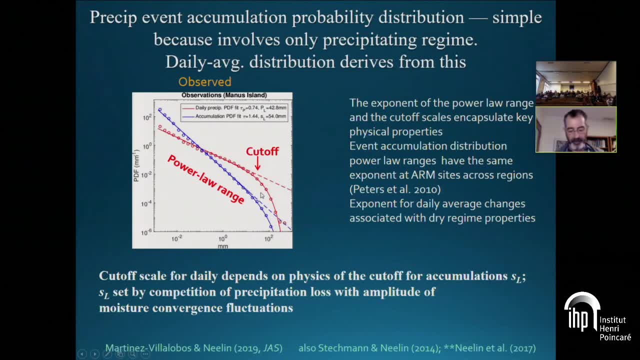 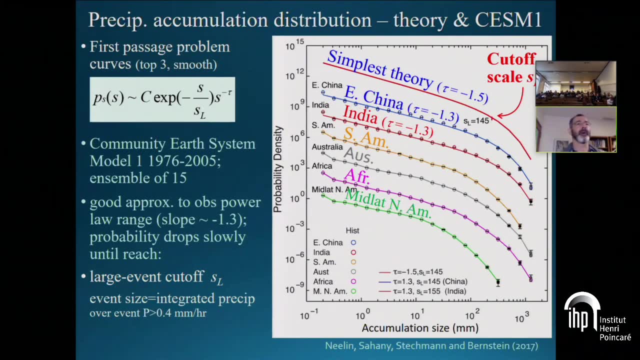 And then we'll give it some consequences of that And that will get inherited right through all of the averages. Okay, so here's an example of looking at accumulations in a climate model. This is from 2017 study. The simplest theory, where you just say your precipitation has an on off switch, gives you a very 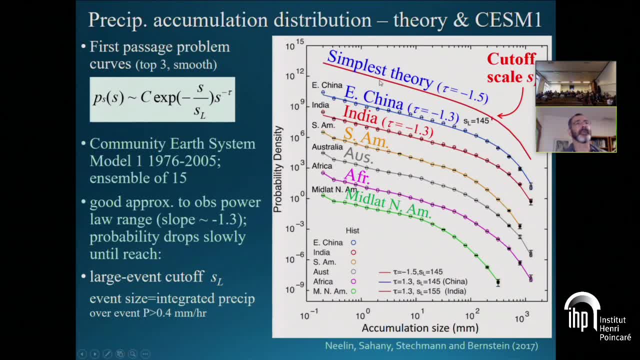 simple first passage process for which the exponent is negative 1.5. when you have the ramp function in the stochastic model It comes down to around negative 1.3, which matches what you get from the full community versus system model fairly well shown for different regions here, in each case with a roughly exponential drop off above a cutoff scale. 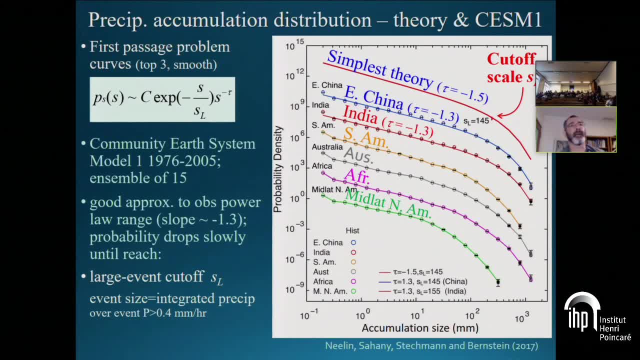 That cutoff scale is given by the competition of the moisture convergence against the precipitation loss. So as you go to a future climate with higher moisture, you expect that scale to be less than 2.5 and it comes down to around a negative 1.3.. 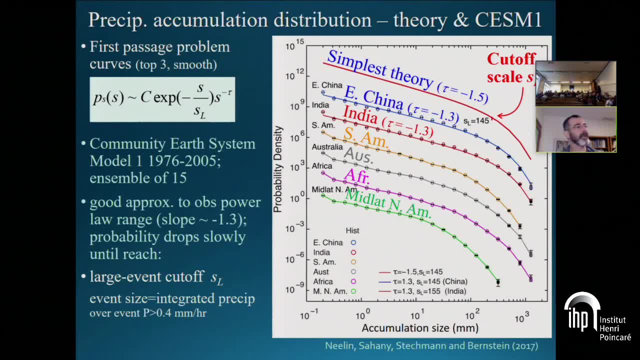 And it's a pretty good example of that, And it's a very good example of that to extend. but I should say that there, if there are dynamical effects like a change in the, in the amount of convergence that you get, that goes into that exact same scale. so you've got a very simple situation. just one thing. 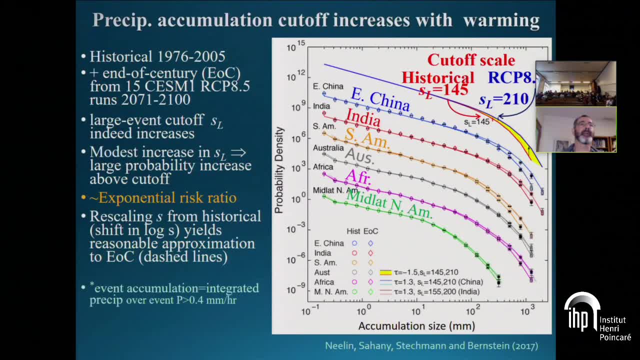 changes. so if we do the experiment of running the climate model in the greenhouse warming scenario again, representation: representative concentration pathway 8.5, end of century- you find that essentially the accumulation size scale rescales. you move your cutoff scale out a little bit so you drop less quickly, and this is on a log scale, so a factor of 10 is shown. 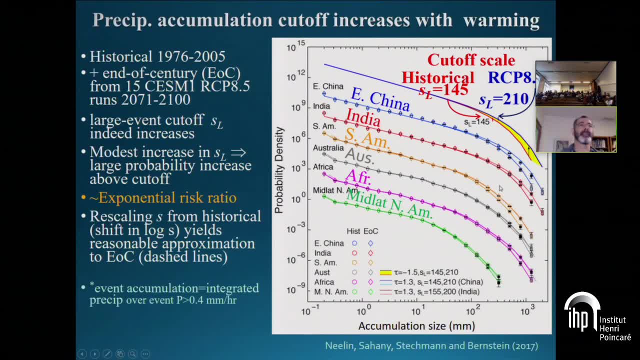 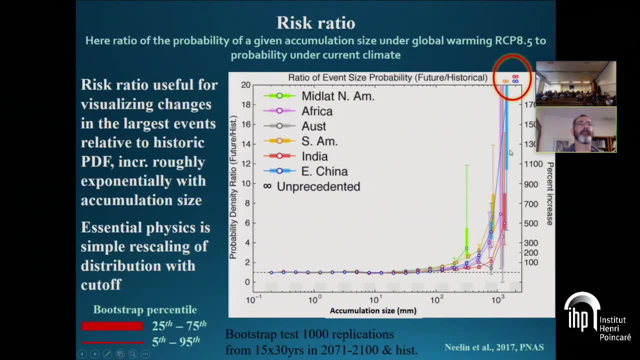 by this arrow here. so you're getting fairly large changes in the extreme events and in fact if you do a risk ratio it goes up awfully exponentially and can reach, you know, thousand percent increase in the very largest event in the climate model projections. does this occur in? 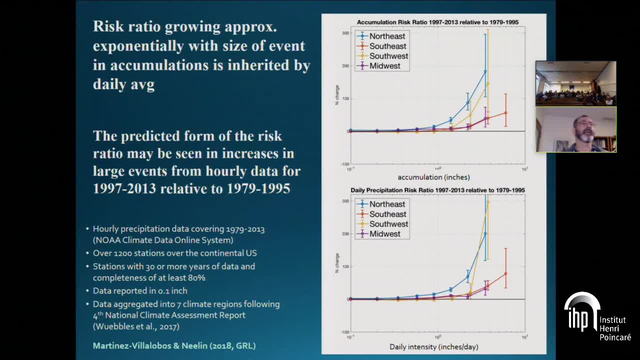 observations: yes, this is looking at the US hourly data sets forming accumulations and this is the risk ratio for accumulations for certain regions shown above, and then the daily precipitate in precipitation intensity, with ratios shown below for two sort of decade and a half periods in the more recent period relative to an earlier. 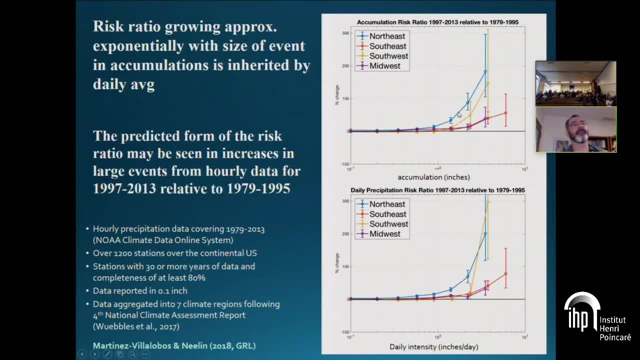 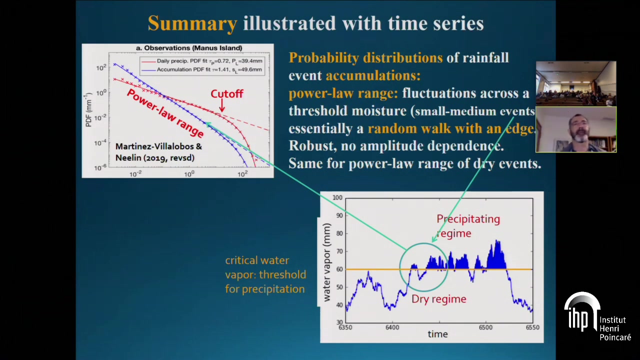 period and, without attribution of this, you can say that when you do have this type of change, it follows the form that we have been arguing for, with this approximately exponential increase over time in the risk ratio. okay, so let's let's summarize graphically some of the 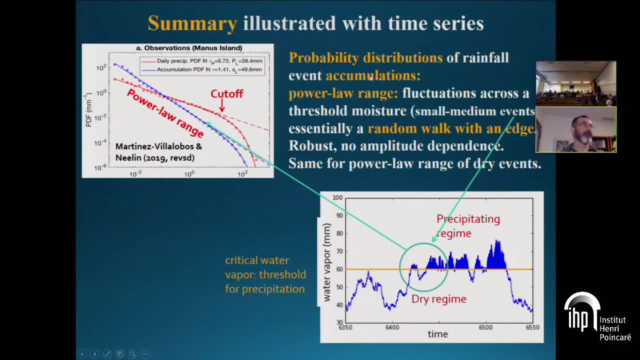 dynamics. that's going into this. first of all, for this probability distribution of precipitation, the power law range in the accumulations is coming simply from in in the, as you're moving, as your dynamics is changing, your water vapor, you reach a threshold where you can begin to precipitate, schematized by these filled in blue areas here in this. 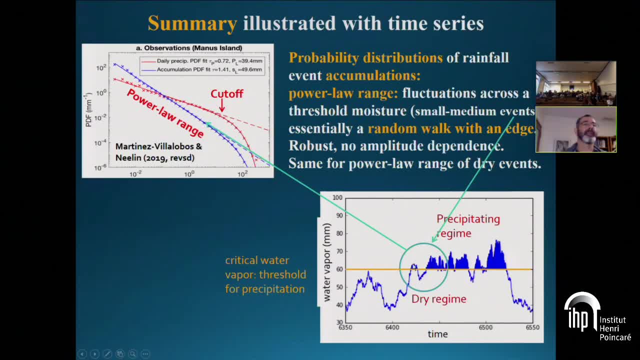 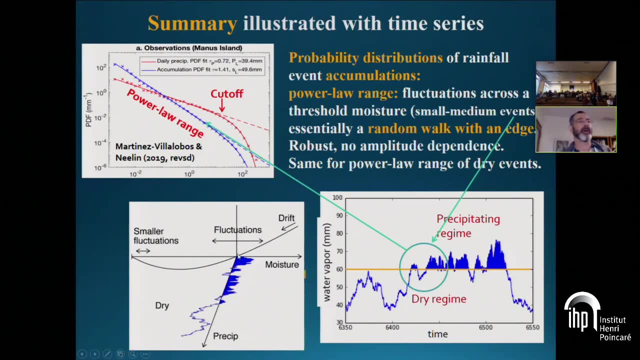 time series of the water vapor and you're going to tend to fluctuate back and forth across this threshold. if i illustrate this as a random walk, with the time axis coming out here. once you're running up this way, your random walker is wandering back and forth across this threshold. say, this is up on a sidewalk. 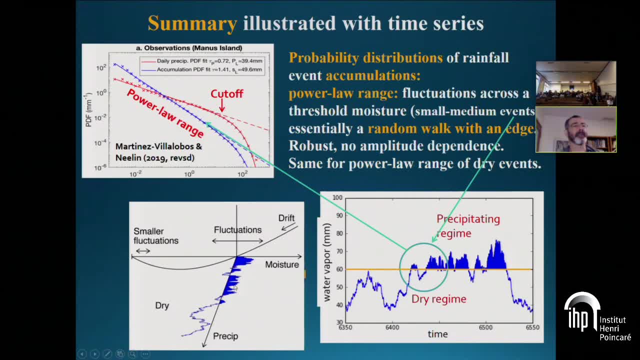 and this is down in the ditch. the up on the sidewalk is the raining regime, the down the ditch is the dry regime, the the random walker will stagger back and forth across this. the pdf of the water vapor value relative to that threshold will tend to increase as time to the half. 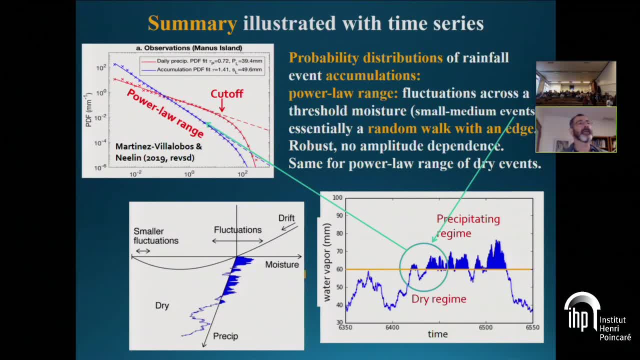 if you're moving forward in the simplest possible case, and so the flux across this will go, like that time, to the negative 1.5, and of course it's not quite time. it's the accumulation of the, the accumulation of the rainfall, that's your true measure of the. 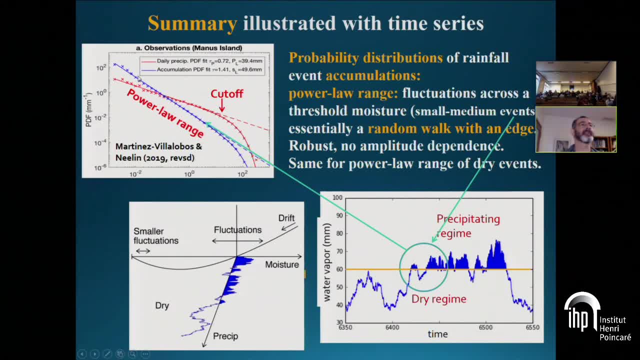 passing time in each of these events. but anyway, that gives you this steep, roughly one minus 1.5 range here in the simplest case, and then when you get to, and that's quite robust, it doesn't have any amplitude dependence on your um, your parameters, and it tends to stay the same from. 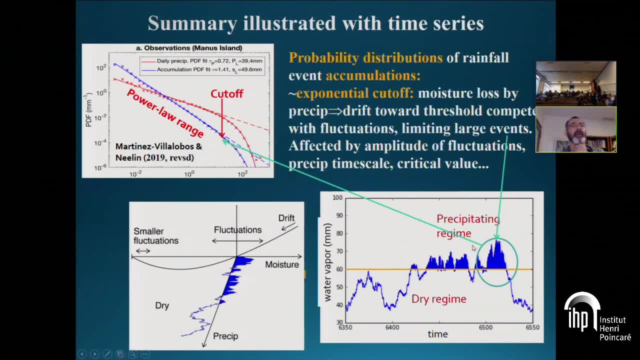 regime to regime. when you're talking about the cutoff, uh, if your precipitation that you've rained out during events is growing with time, that will continue to grow. that's initially a slower growth because it's scaling, in the simplest case, like time. if you had an 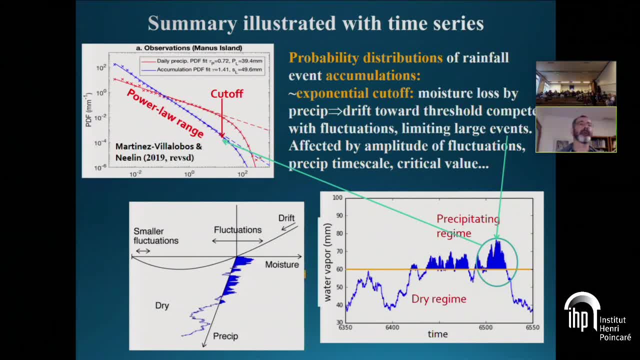 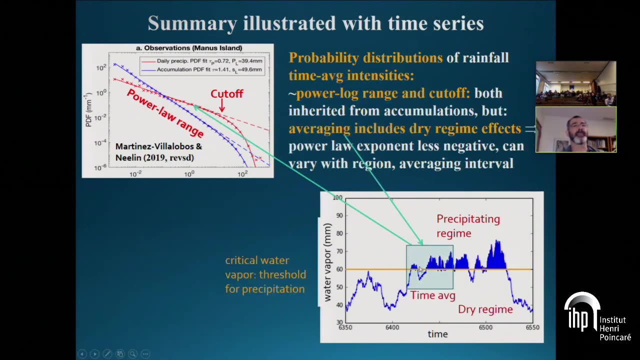 even precipitation rate, and so it will come into play uh later in the event. so for the larger events and will yield this cutoff that balances the precipitation loss against the moisture fluctuations. when you do a time average, you're simply taking a number of these events and adding them up together. you reduce the um, the num, the probability of a small amount in that. 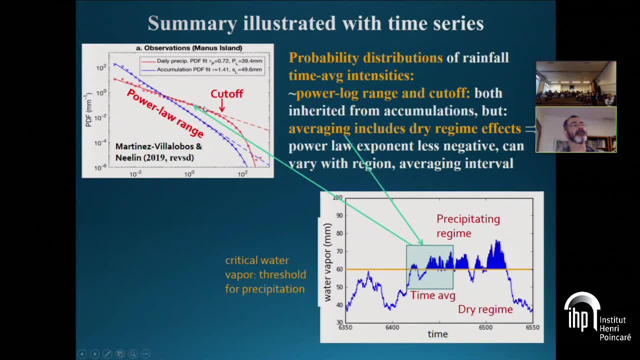 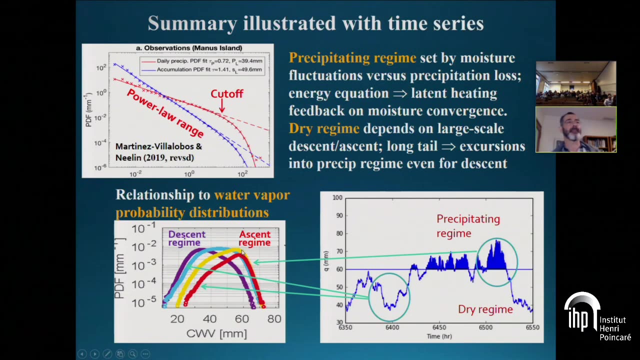 averaging window increase the probability of a large event in this range here. but the cutoff has the same physics and is inherited from what we had in the accumulations. and then, if you think back to the relationship to the thermodynamic environment here, um, what's going on in the precipitating regime is dominated by that precipitation physics and is thus 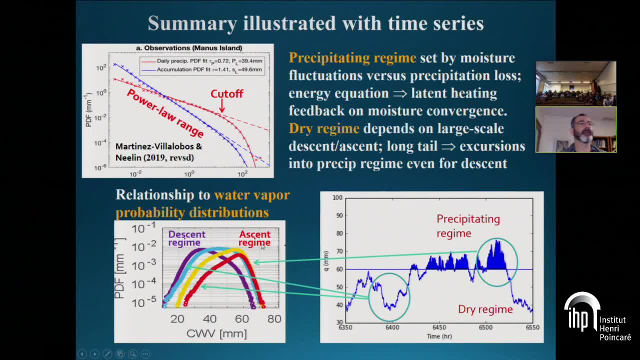 relatively simple and relatively similar whether you're in a large-scale ascent regime or a large-scale descent regime from a climatological point of view, whether you're being driven by negative net fluxes in the column or negative net fluxes into the column. but you will, when you exit the precipitating regime, you will obey different dynamics. 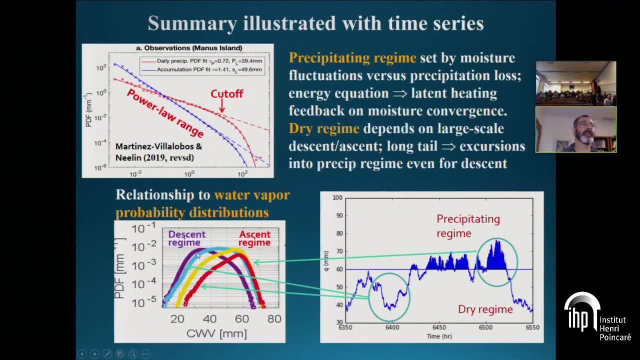 with the large scale ascent. the descent regime will have a peak at low water vapor although, as we saw, it has this fairly slow drop until you hit the precipitating regime. so you still sometimes get uh precipitation, even in a in a dry zone uh, and then in the uh convergence regime we're going. 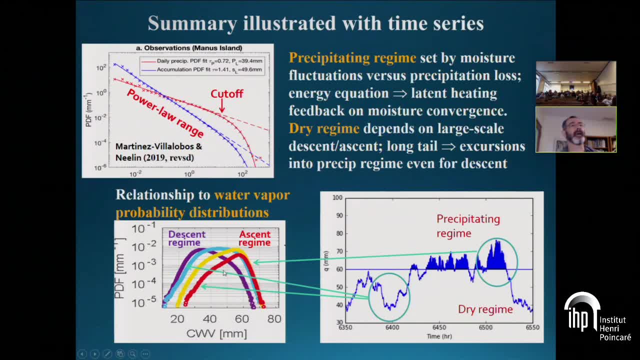 to see what the precipitation water level is now. uh, in the secular regime you're just really ahuing down into the precipitating режим, low level convergence regime. you're just returning yourself more expeditiously into the precipitating regime when you're wandering around in the dry. 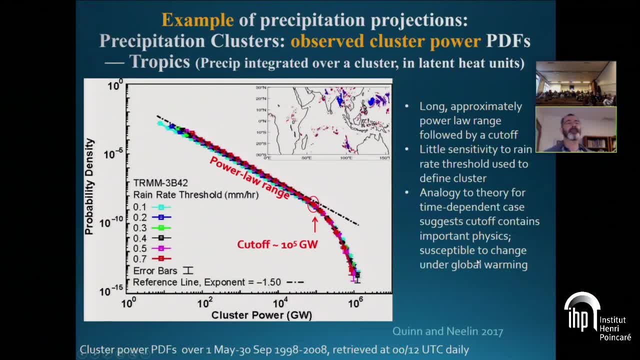 regime. you have a a drift upwards towards the onset um the to. that returns you there. okay, four, two below here we're good maximum temperature when we exit the time attendance regime. look used on the Coffee's. you look, wipe out Suffering Ours. Theぐas Exp. kim accommodates 67%. look over. 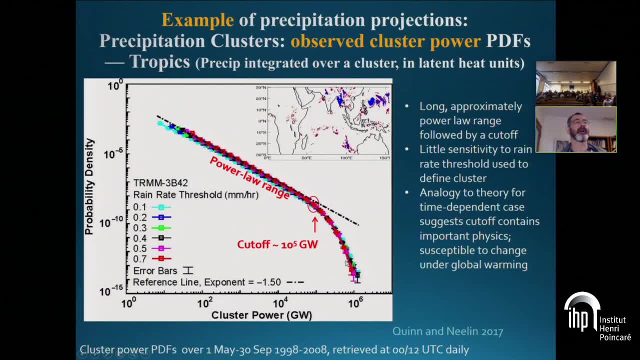 at regular time conditionless. H shouldn't download on Mon балян again in a log log plot of the probability of measure of the cluster precipitation. this cluster power is just the precipitation integrated over a contiguous precipitation cluster and when you look at the smaller clusters they have a roughly power law range. again, the exponent is: 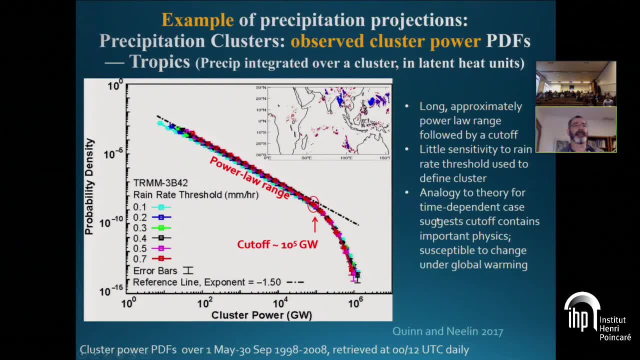 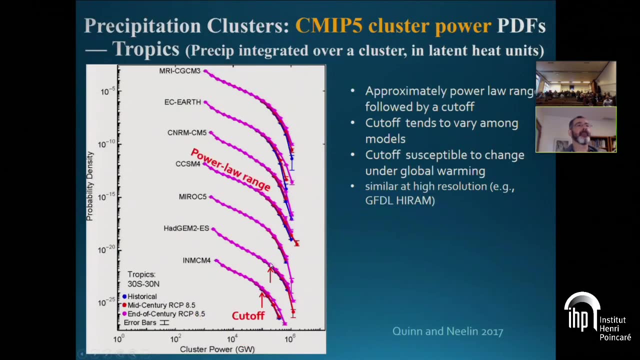 around minus 1.5. so you are tempted to think that there must be an analogy of theory for the time dependent case, you would suspect that the cutoff contains important physics and that it would be susceptible to change under global warming. if you look in a series of climate models here the pdfs- 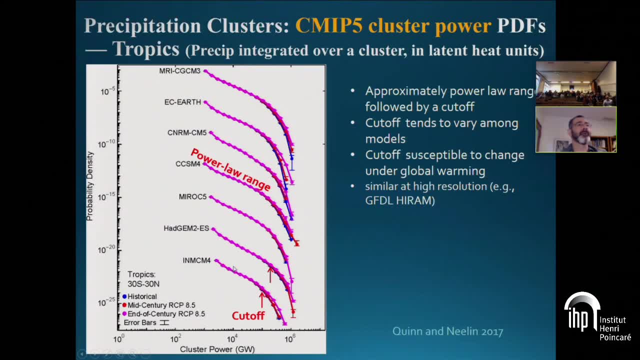 of the cluster power are being shown separated by two decades, just so that you can see them. so we're shifting them up as we go along, but you can compare the slopes. in each case you have a range which is roughly power law, roughly in the range of minus. 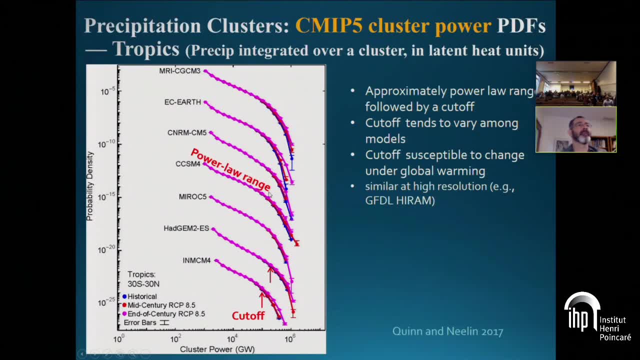 1.5 exponent followed by a roughly exponential drop. if you look at the blue is historical versus end of century is purple. you tend to have an extension of this cutoff and thus an increase in the probability of the various largest events and indeed that tends to have a roughly exponential. 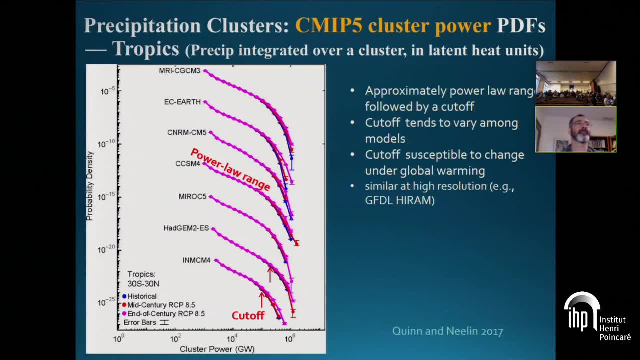 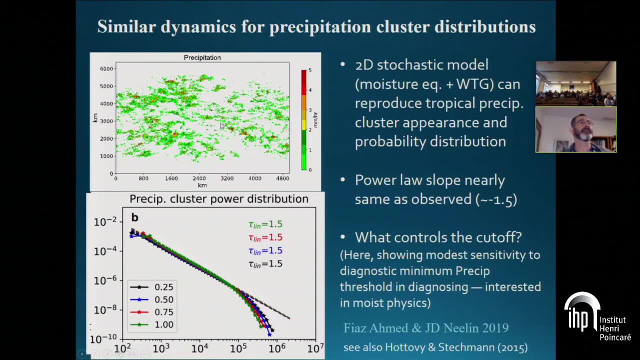 increase in the risk ratio with the size of the events. so can we do this in the stochastic model? this is an example of a snapshot of precipitation from a two-dimensional version of the stochastic model. in the box there's a slight large-scale convergence driven by fluxes in here and a slight descent out here, so it's like a very gentle hadley cell. 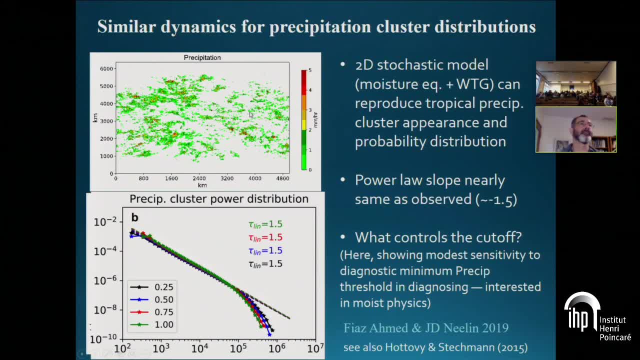 and they're stirring by a stochastic, purely rotational flow, as well as the the tickling of the divergence, as we saw in the earlier equations, and then feedbacks of the divergence in the precipitation, because we're in a we have a weak temperature gradient energy equation that gives that feedback. 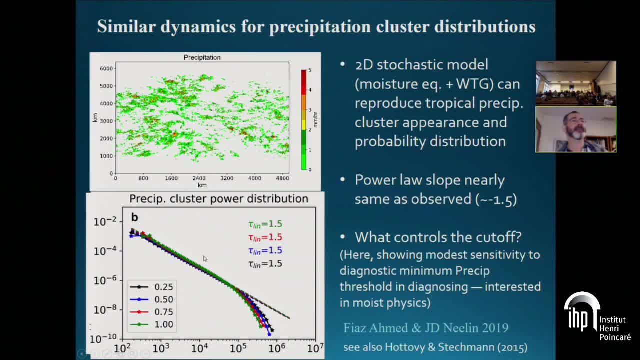 as we saw before. so do we get the cluster power distributions? yes, about a minus 1.5 long power law range followed by a cutoff. here is just testing the sensitivity of the cutoff to the thresholds of the precipitation. and then we're interested in what moist physics would govern this. 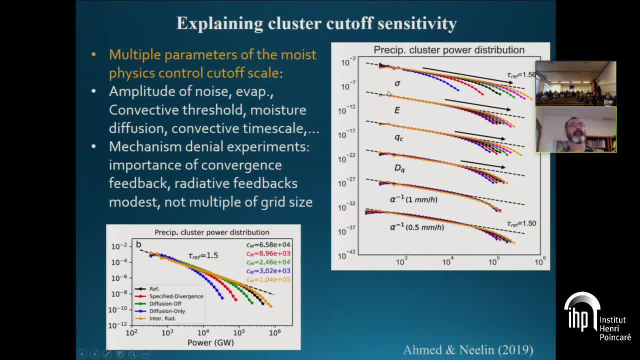 so it turns out, yes, the cutoff depends on moist physics. you can do a series of parameter perturbation experiments with things like the amplitude of the noise, the evaporation, the critical value at which the precipitation increases the diffusion, the time scale of the, the precipitation loss rate and, in. 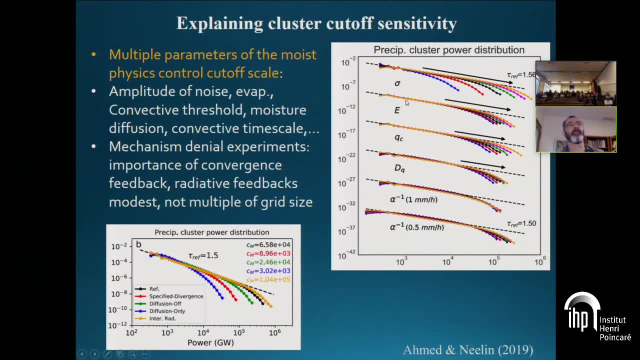 in each case you find that the power law range stays about the same and the cutoff tends to change. And then you can furthermore do experiments where you mechanism denial experiments. for instance, you have or don't have interactive radiation that has a modest effect. where you 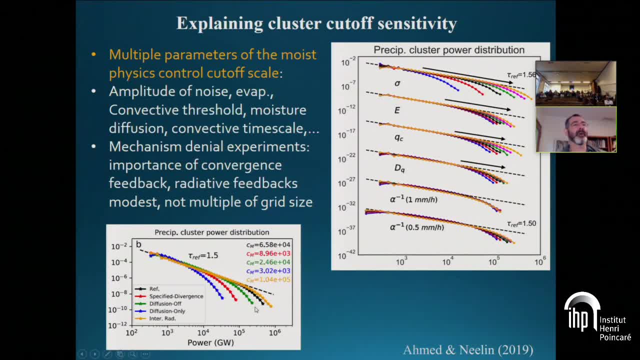 switch the diffusion off, that has some effect. where you take out the specified divergence instead of feedback. that has a large effect And essentially you have multiple aspects of the moist physics that is going into that cutoff scale. So it's of interest to see if you can. 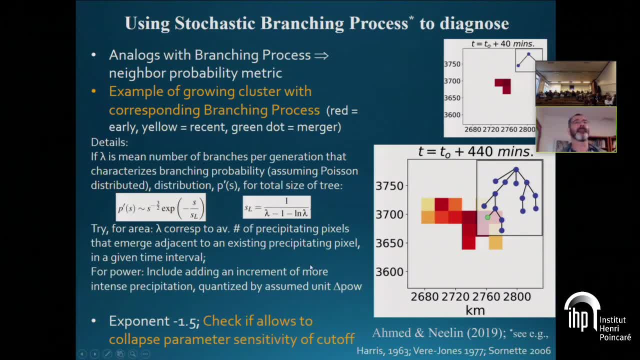 make sense of that multiple dependence on the moist physics you've established. the cutoff scale is important. it's the thing that changes What's a very simple process that we could use to represent this. the stochastic branching process is attempting analog, because if you start with one precipitating cluster, it can add: 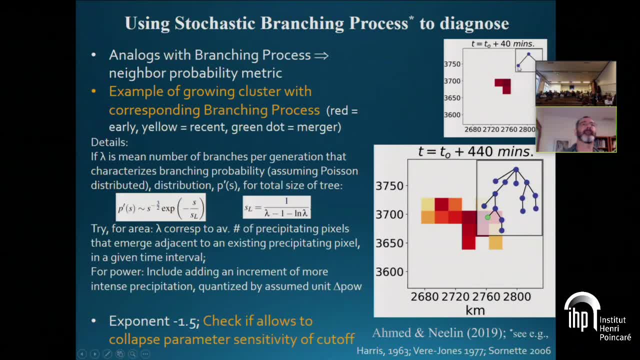 neighbors in the next time step, corresponding to a probability of generating branches in a stochastic branching process. And if you follow forward by units of time, you keep adding clusters, keep adding points to your cluster or losing them. that corresponds to a stochastic branching process. 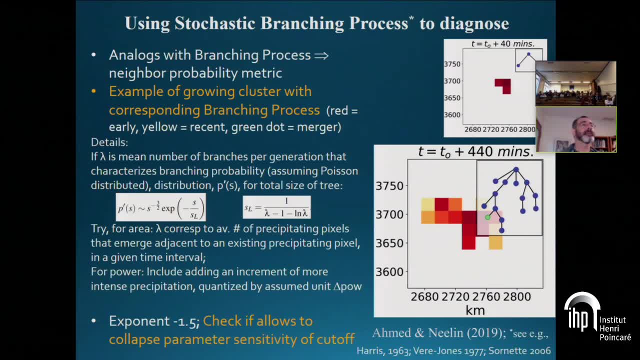 tree Moving forward in time. So if you grab an example that seems relevant, the mean number of branches per generation that you is the important parameter, And if these are Poisson distributed, then the probability distribution for your stochastic branching process would be the size to the negative. 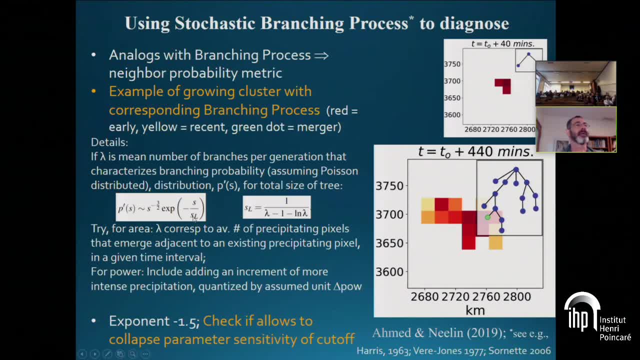 three halves, which is the correct exponent for our parallel range, And then an exponential drop with a scale that is given in terms of that mean number of branches. So then you jump in, you diagnose for a given run of your model, measure of how many pixels you tend to add to your cluster per time, step for a growing. 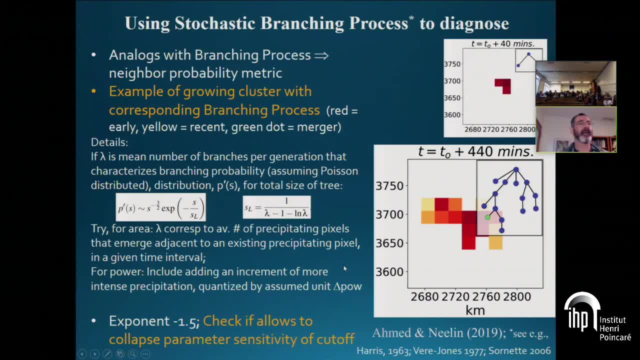 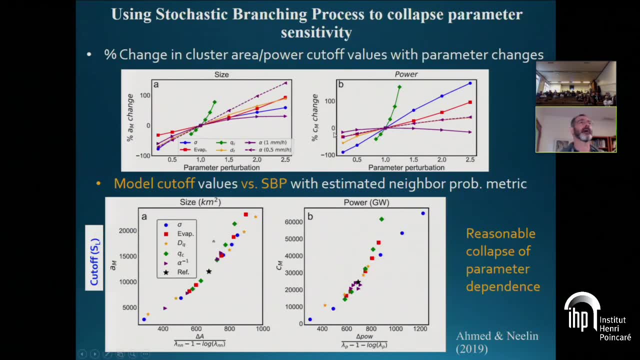 cluster And then we want to check if that helps us any with the parameters sensitivity. can we collapse that? So in the top the four dashed log here. if I go back one step, this is our parameter perturbation relative to a reference value. This is the percent change in the cluster area and the 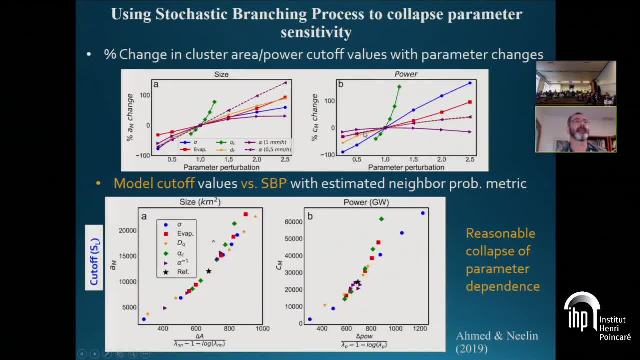 excuse me, I have to go back one slide cluster area and the cluster power, the integrated precipitation. So that's the raw input. If we instead display the X axis as being this cutoff scale that we expect from the branching process, what we find is that, to a reasonable rate, we're going to be able to use this interaction from a. 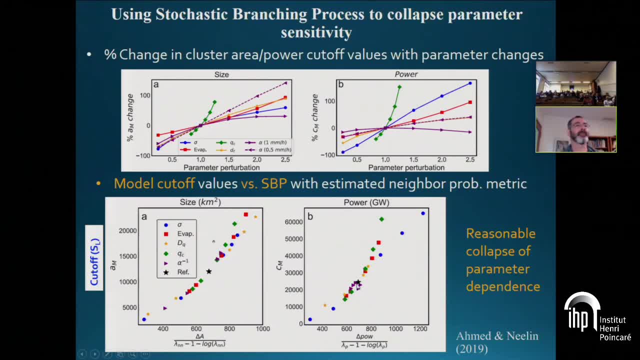 we're going to be able to use this interaction from a belly-to-тов belly-to-top data belly-to-top data. we're going to be able to use this interaction from a extent, for both the area and the power we collapse onto, a single dependence for. 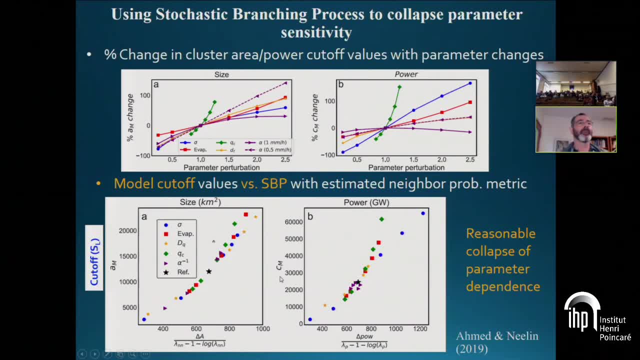 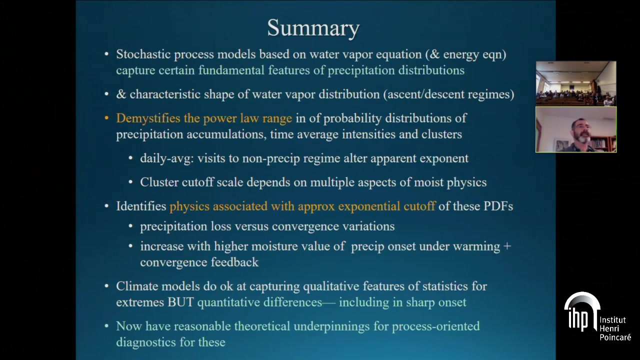 all the parameter perturbation. so what this says is that, yes, the cutoff scale is important. it depends on various aspects in those moist physics, but you can boil it down into what's the probability of generating new neighbors once you start conducting. okay. and that brings me to my summary and essentially. 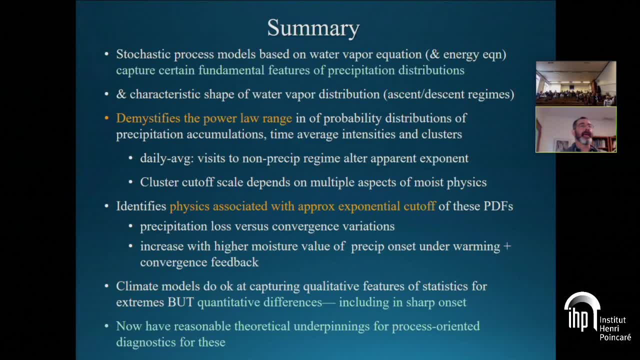 your stochastic model helps you with several things. it demystifies the power law range that you see in the probability distribution of precipitation, both accumulations and time average intensities. it establishes the relationship between those two probability distributions. it gives you moist physics associated with the probability distribution of the 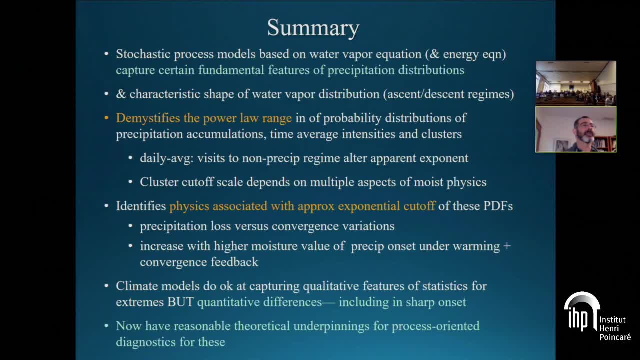 precipitation, both accumulations and time average intensities. it gives you the roughly exponential cutoff of these distributions and it tells you the relationship to the thermodynamic environment as you move around in water vapor and by complex dynamics which we've here represented as stochastic. so at this point we have reasonable theoretical underpinnings for the 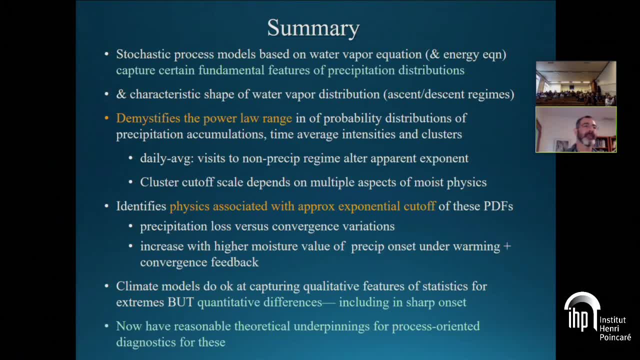 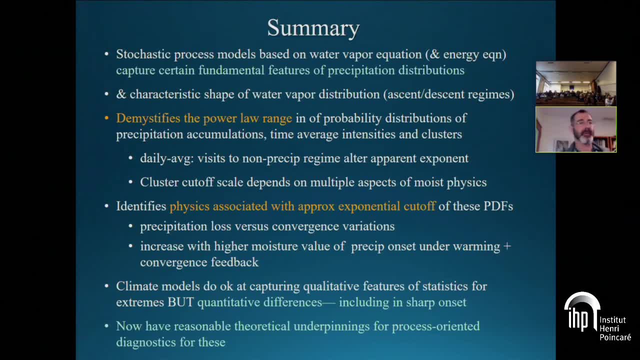 the previous slides and we've shown you in the previous slides and I the previous slides and we've shown you in the previous slides and I think I'll stop there see if there's time for think. I'll stop there, see if there's time for think. I'll stop there see if there's time for questions. yeah, thank you very much. 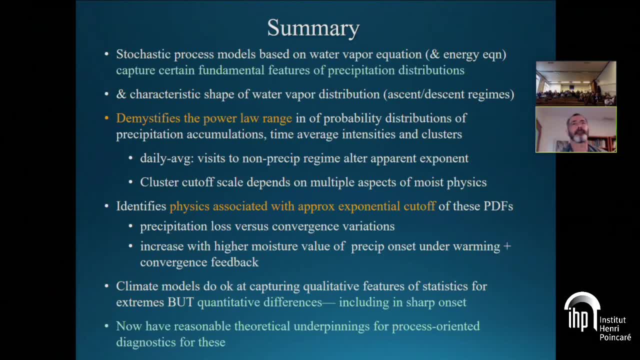 questions. yeah, thank you very much. questions. yeah, thank you very much, David. we have a few minutes for questions from. we have a few minutes for questions from. we have a few minutes for questions from the audience. Michael, you should use a microphone. Michael, you should use a microphone. 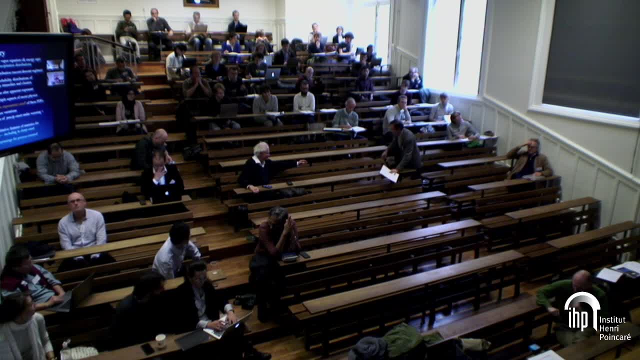 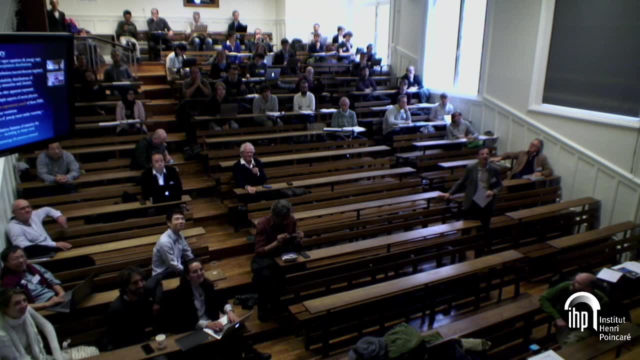 Michael, you should use a microphone, otherwise he won't understand, otherwise he won't understand. Michael, you should use a microphone, otherwise he won't understand, otherwise he won't understand. hi, David, good to see you, even from a. hi, David, good to see you even from a. hi, David, good to see you even from a distance. Michael, I can. I can't quite see. 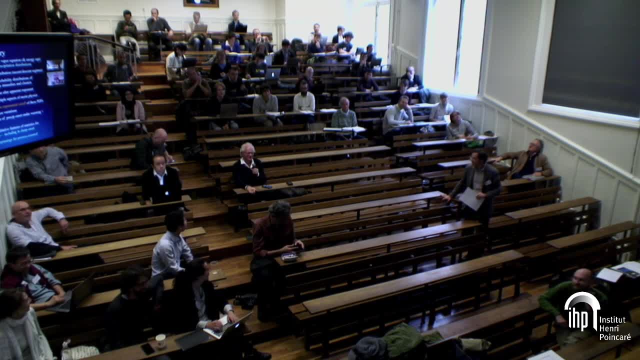 distance, Michael, I can. I can't quite see distance, Michael, I can. I can't quite see you, but I can recognize your voice. yeah, you, but I can recognize your voice. yeah, you, but I can recognize your voice. yeah, well, these go well one way, but not the. 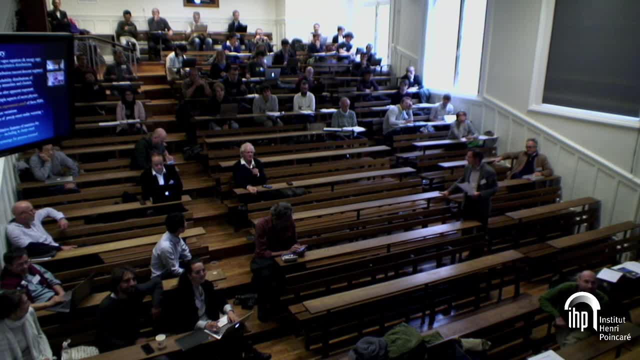 well these go well one way, but not the well these go well one way, but not the others so well, to the extent I mean this. others so well, to the extent I mean this, others so well. to the extent I mean this was pretty impressive and thank you very. 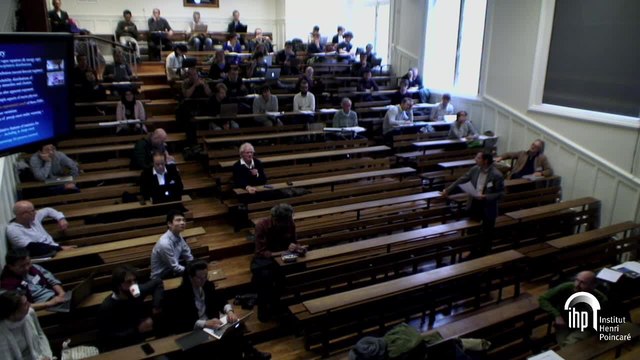 was pretty impressive and thank you very was pretty impressive and thank you very much for taking the trouble. any concrete much for taking the trouble. any concrete, much for taking the trouble. any concrete advice to those poor GCM is about. advice to those poor GCM is about 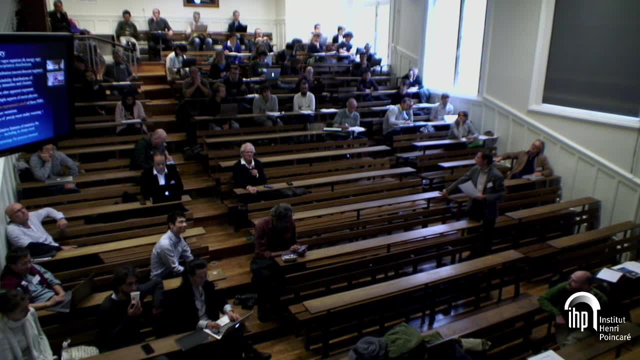 advice to those poor GCM is about how they might improve the pre-safe. how they might improve the pre-safe, how they might improve the pre-safe parameterizations from collapsing all parameterizations. from collapsing all parameterizations, from collapsing all these distributions and finding branching these distributions and finding branching. 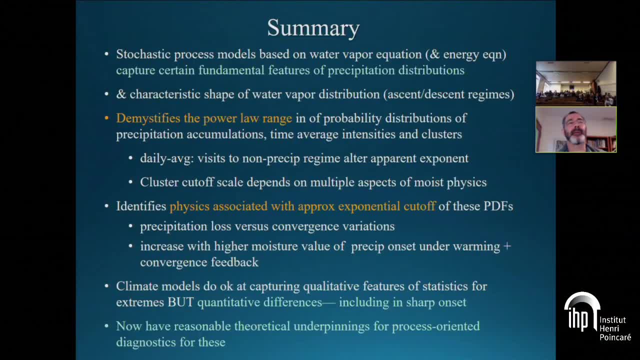 these distributions and finding branching models and stuff. when you, when you get models and stuff, when you, when you get models and stuff, when you, when you get to a particular GCM, you are needing to to a particular GCM, you are needing to to a particular GCM, you are needing to get down into the weeds of the 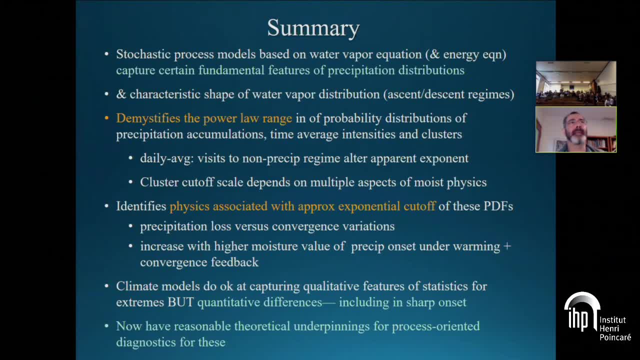 get down into the weeds of the get down into the weeds of the parameterization. one substantial factor is parameterization. one substantial factor is parameterization. one substantial factor is the representation of entrainment, and that, the representation of entrainment, and that the representation of entrainment, and that was the the, the thing that I 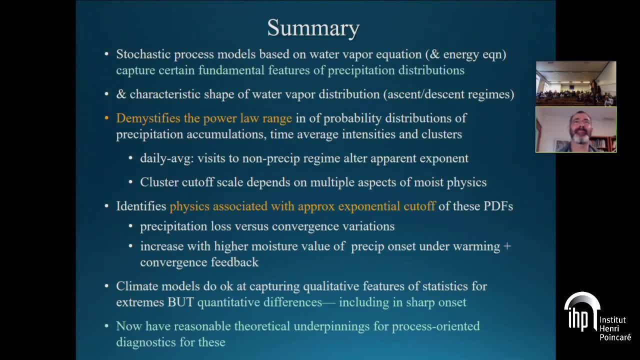 was the, the, the. the thing that I was, the, the, the. the thing that I summarized in one slide in order for the. summarized in one slide in order for the. summarized in one slide in order for the. for this talk, I wanted to emphasize the. for this talk, I wanted to emphasize the. 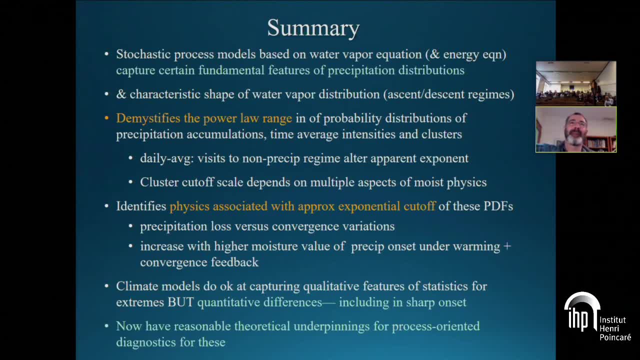 for this talk. I wanted to emphasize the stochastic modeling and the. the stochastic modeling and the. the stochastic modeling and the. the explanations arising from that that one. explanations arising from that that one. explanations arising from that that one. slide summary of what sets the onset is. slide summary of what sets the onset is. 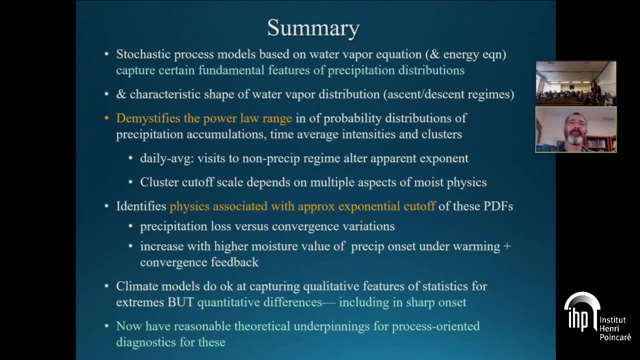 slide summary of what sets the onset is one of the things that you most need to, one of the things that you most need to, one of the things that you most need to take apart when you're looking at what a take apart, when you're looking at what a. 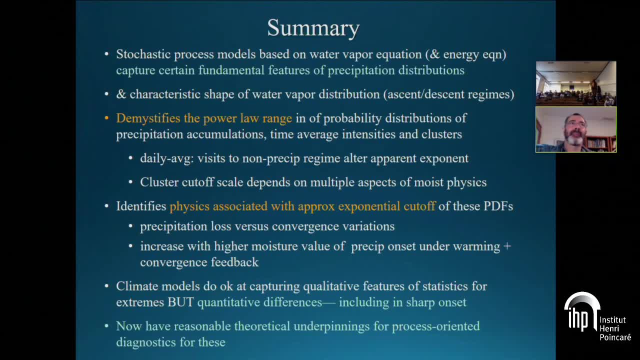 take apart when you're looking at what a stochastic model gives you is the stochastic model gives you is the stochastic model gives you is the examples with CSM of pulling out the examples with CSM of pulling out, the examples with CSM of pulling out the piece of the convective parameterization. 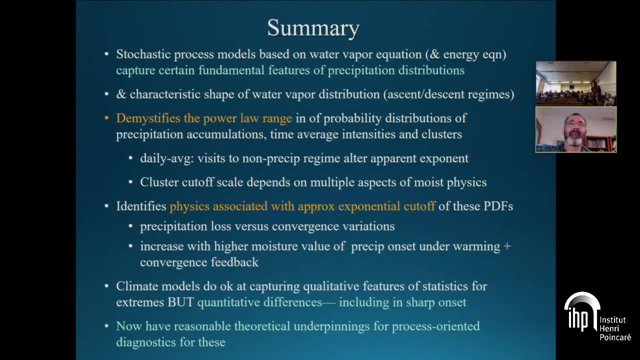 piece of the convective parameterization. piece of the convective parameterization that that does the conditional. that that does the conditional. that that does the conditional instability computation for the plume, instability computation for the plume, instability computation for the plume and looking in detail at the dependence. 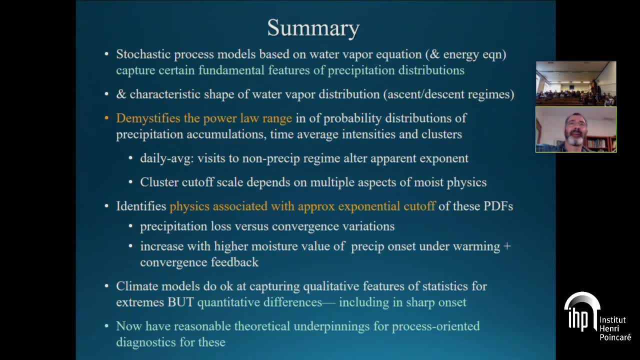 and looking in detail at the dependence and looking in detail at the dependence of that, and that's an example of the of that, and that's an example of the of that, and that's an example of the sort of sort of sort of, when you want to map this onto the 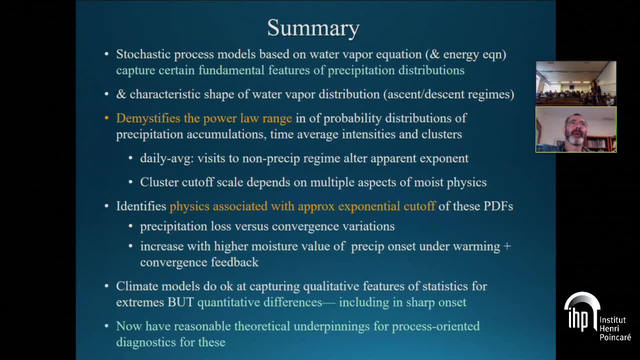 when you want to map this onto the, when you want to map this onto the graphic details of the parameterization, graphic details of the parameterization, graphic details of the parameterization, what you need to do, what you need to do, what you need to do. but I think the stochastic model gives. 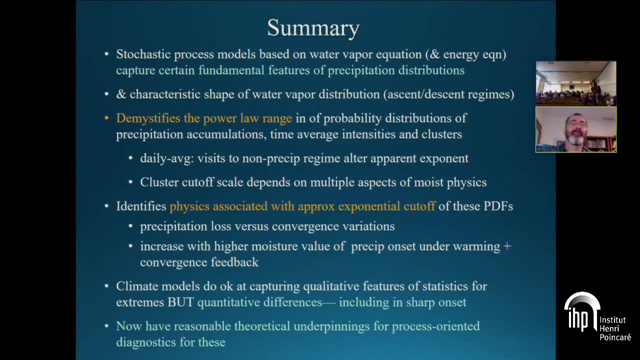 but I think the stochastic model gives. but I think the stochastic model gives you all the pieces that you need to you, all the pieces that you need to you, all the pieces that you need to understand how these things understand, how these things understand how these things relate to each other. and so, for instance, 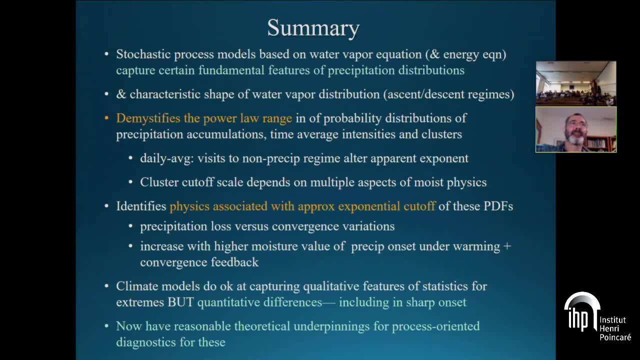 relate to each other and so, for instance, relate to each other. and so, for instance, if you're, if you're, if you're worried about your, worried about your, worried about your high-end precipitation and its high-end precipitation and its high-end precipitation and its probability distribution. 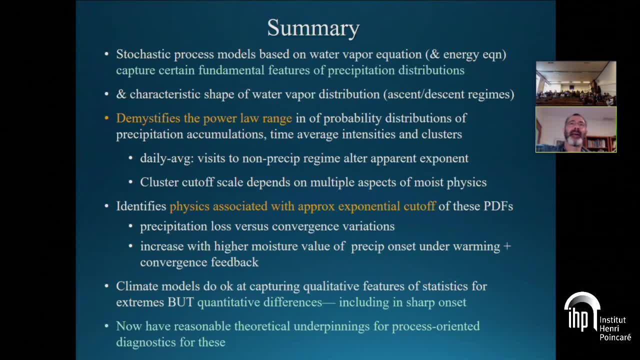 probability distribution. probability distribution not being strong enough, not being strong enough, not being strong enough- that you're looking at in your code, that you're looking at in your code, that you're looking at in your code. good, great, thank you very much. and hope. good, great, thank you very much and hope. 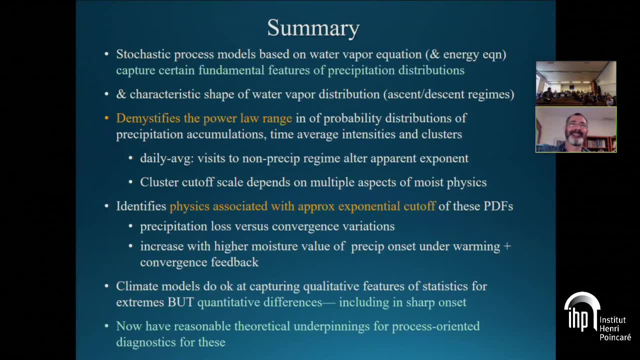 good, great, thank you very much and hope to see you soon. to see you soon. to see you soon. okay, great thanks. okay, great thanks. okay, great thanks. thank you, michael. thank you, david, any. thank you, michael. thank you, david, any. thank you, michael. thank you, david. any other question from the audience? 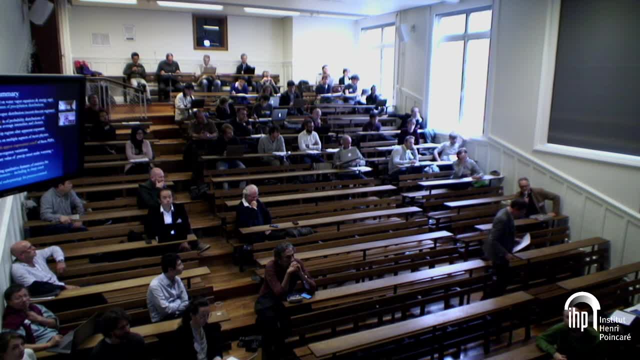 yeah, hi, hi, david, it's roberto buizza. i yeah, hi, hi, david, it's roberto buizza. i- yeah, hi, hi, david, it's roberto buizza. i was at the european center. till was at the european center. till was at the european center till one year ago. i'm sorry, i'm having a. 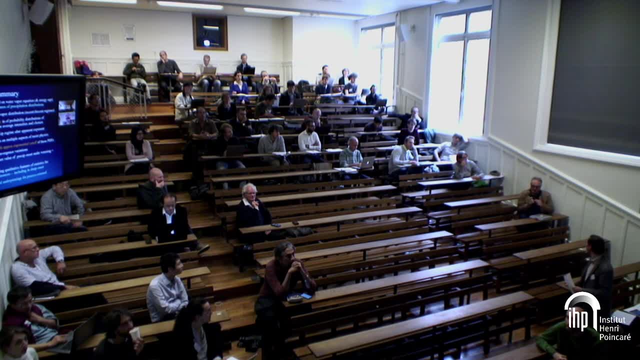 one year ago. i'm sorry i'm having a one year ago. i'm sorry i'm having a little trouble hearing. okay, roberto, little trouble hearing. okay, roberto, little trouble hearing. okay, roberto, buizza. can you hear me, buizza? can you hear me, buizza? can you hear me? can you hear me? hello. 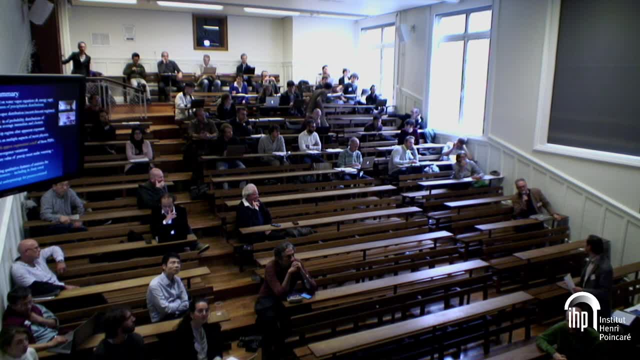 can you hear me hello. can you hear me hello? yes, i can hear now just okay, so it's yes, i can hear now just okay, so it's yes, i can hear now, just okay. so it's roberto buizza from the. roberto buizza from the. 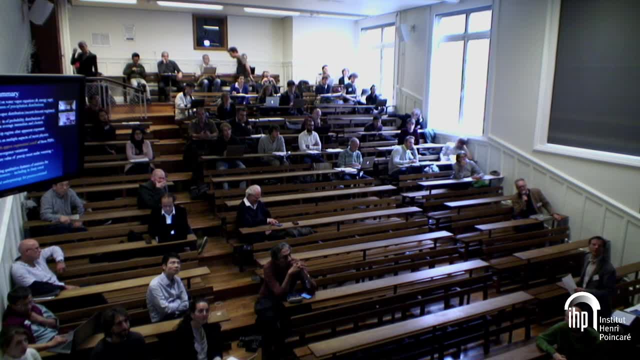 roberto buizza from the formerly european center, formerly european center, formerly european center: hi, okay. so what i want to say is a hi, okay. so what i want to say is a hi, okay. so what i want to say is a comment on the actual resolution of these. 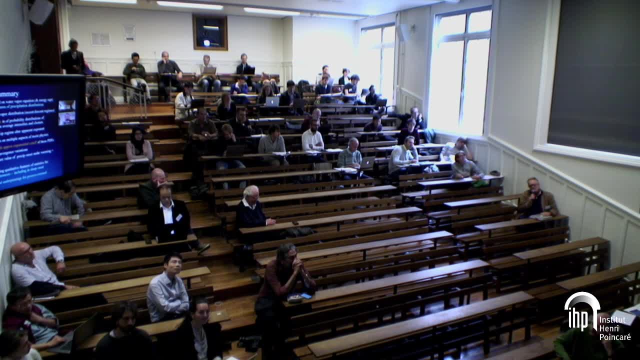 comment on the actual resolution of these. comment on the actual resolution of these gcms, gcms, gcms, and uh, we don't we, we shouldn't forget, and uh, we don't, we, we shouldn't forget, and uh, we don't we, we shouldn't forget that the with the resolution delta x. 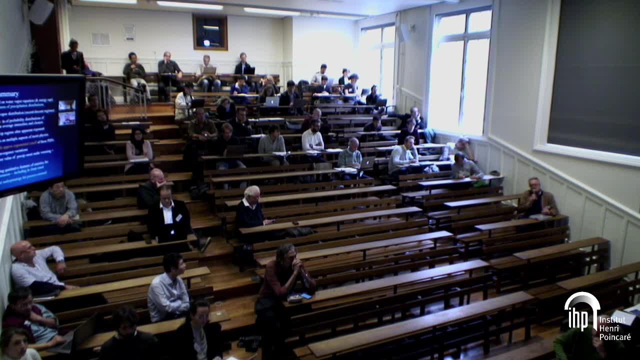 that the with the resolution delta x, that the with the resolution delta x, actually what the gcms are able to, actually what the gcms are able to, actually what the gcms are able to resolve, are, roughly speaking, five times resolve, are, roughly speaking, five times resolve, are, roughly speaking, five times the grid. 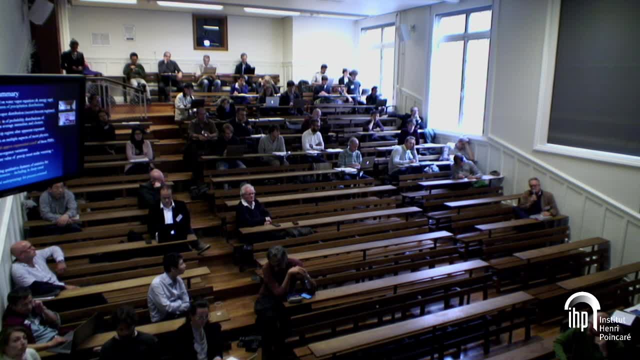 the grid, the grid resolution. so, if we're talking about resolution, so if we're talking about resolution, so if we're talking about models used for climate studies, models used for climate studies, models used for climate studies, the models are now have a resolution of. the models are now have a resolution of. 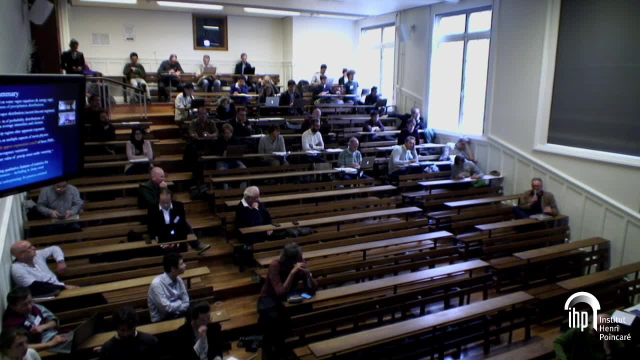 the models are now have a resolution of about 50 to 100 kilometers, which means about 50 to 100 kilometers, which means about 50 to 100 kilometers, which means that they have, they are capable to that, they have, they are capable to that they have, they are capable to actually. actually actually resolve, resolve. resolve: scales only at down to 200- 200 kilometers. scales only at down to 200- 200 kilometers. scales only at down to 200- 200 kilometers or so or so or so. if we're talking about weather models: no. if we're talking about weather models: no. 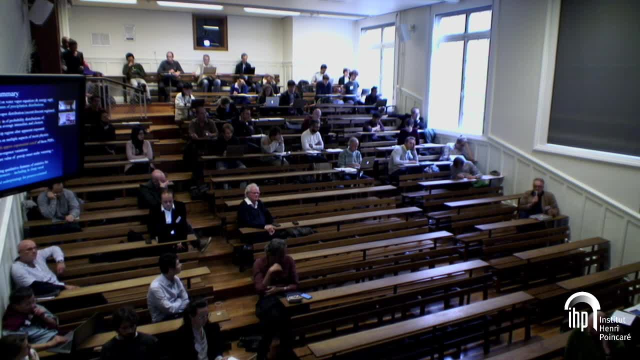 if we're talking about weather models. no, they are running now at about. they are running now at about. they are running now at about. two to ten kilometer resolution, again a two to ten kilometer resolution, again a two to ten kilometer resolution, again. a factor of five will bring you to 10 to 50. factor of five will bring you to 10 to 50. factor of five will bring you to 10 to 50 kilometer actual resolution. what i mean kilometer actual resolution. what i mean kilometer actual resolution. what i mean actual resolution? i mean that the model. 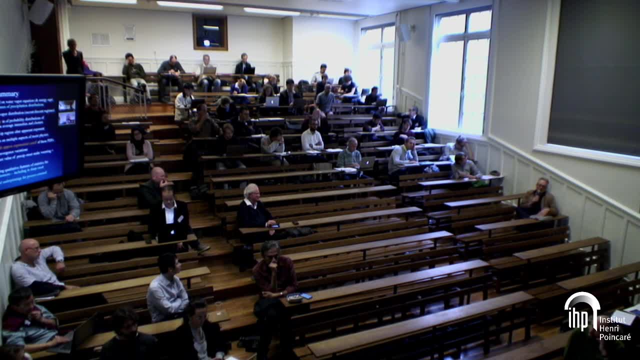 actual resolution. i mean that the model actual resolution, i mean that the model spectra energy spectra is similar spectra energy spectra is similar spectra energy spectra is similar to the observation spectrum, to the observation spectrum, to the observation spectrum. so when we are trying to judge, so when we are trying to judge, 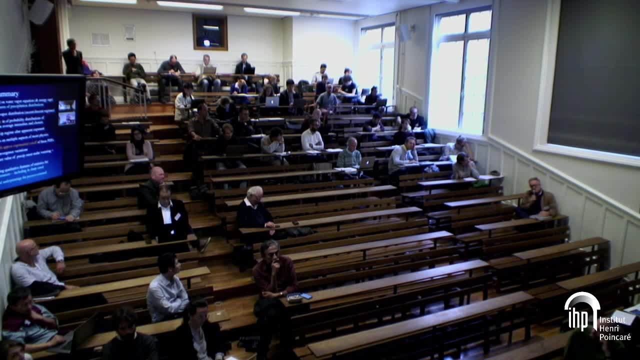 so, when we are trying to judge the quality of the models, in predicting the quality of the models, in predicting the quality of the models, in predicting perceived, perceived, perceived, we should really keep this in mind, the we should really keep this in mind, the we should really keep this in mind- the models. 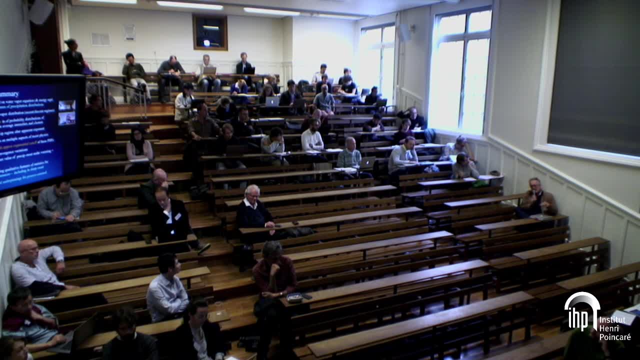 models, models are really trying to simulate precipitation over scales, precipitation over scales, precipitation over scales which are still rather coarse and often which are still rather coarse and often which are still rather coarse, and often we compare, we compare, we compare models, models, we compare models simulation to observations. 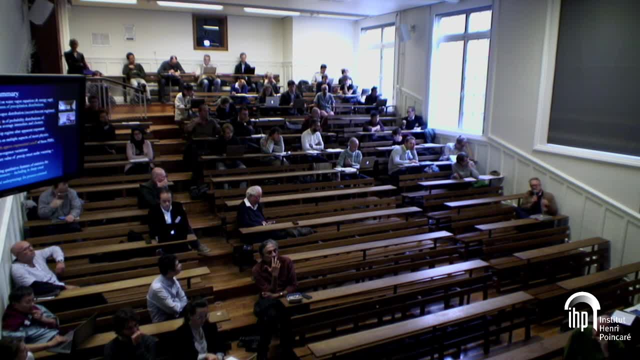 simulation to observations. simulation to observations: sometimes average, but still sometimes average, but still sometimes average, but still. observation captures a lot of very small observation. captures a lot of very small observation. captures a lot of very small details, details, details that the models that we're using now are. 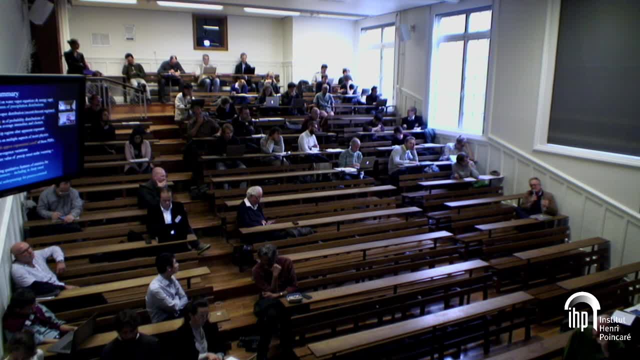 that the models that we're using now are that the models that we're using now are really not capable, really not capable, really not capable to use. so it's very difficult to comment to use. so it's very difficult to comment to use. so it's very difficult to comment on the taste of the distributions. on the taste of the distributions. on the taste of the distributions, one can say much more about. one can say much more about. one can say much more about: low value of precipitation: 10- 20. low value of precipitation: 10- 20. low value of precipitation: 10- 20 millimeters. 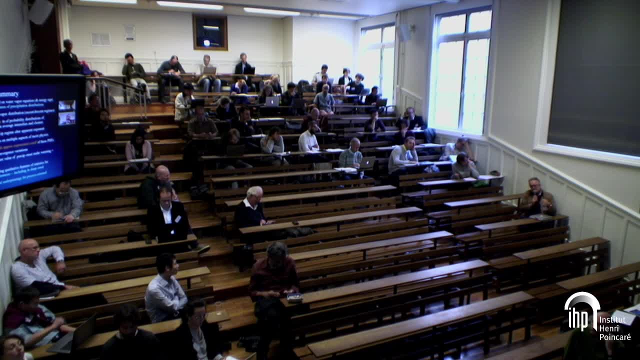 millimeters, millimeters, millimeters, an hour or so, but it's very difficult an hour or so, but it's very difficult, an hour or so, but it's very difficult to say something, to say something, to say something about values higher because the models, about values higher because the models. 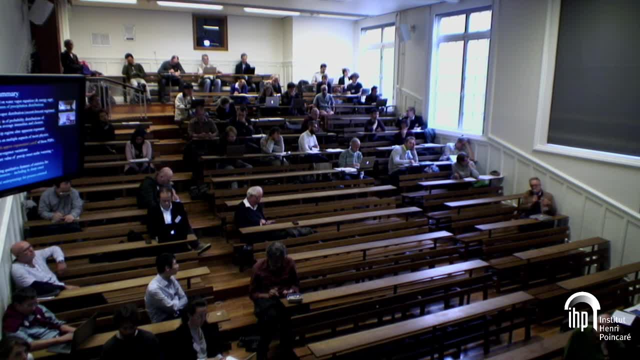 about values higher, because the models are really not yet. there are really not yet, there are really not yet there. despite all what we can do to the, despite all what we can do to the, despite all what we can do to the parameterizations, parameterizations, parameterizations, the scales are not resolved, and i don't. 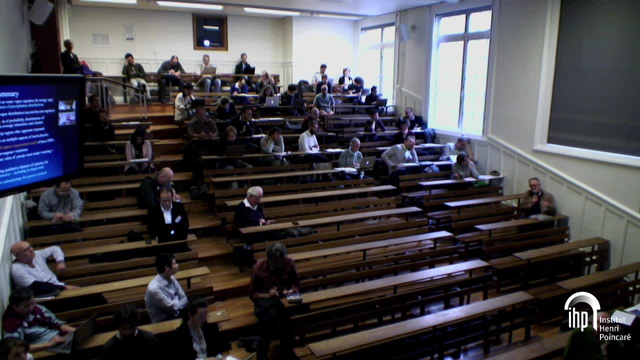 the scales are not resolved. and i don't the scales are not resolved and i don't think that stochastic processes think that stochastic processes think that stochastic processes can actually help us a lot because can actually help us a lot, because can actually help us a lot, because even with stochastic processes, they 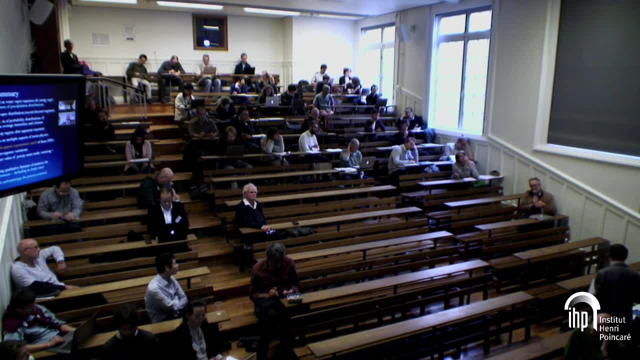 even with stochastic processes. they, even with stochastic processes, they, this case that the models are capable, this case that the models are capable, this case that the models are capable to resolve, remain to resolve, remain to resolve, remain roughly what i said, which is about five. roughly what i said, which is about five. 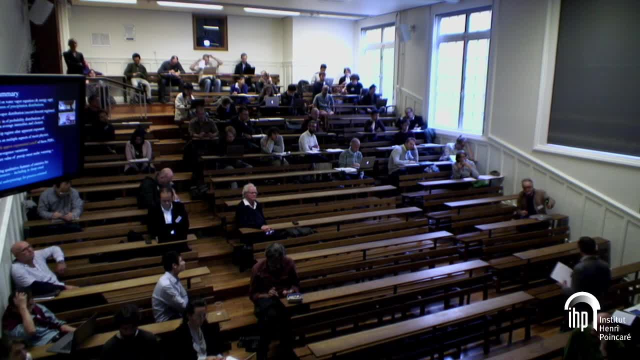 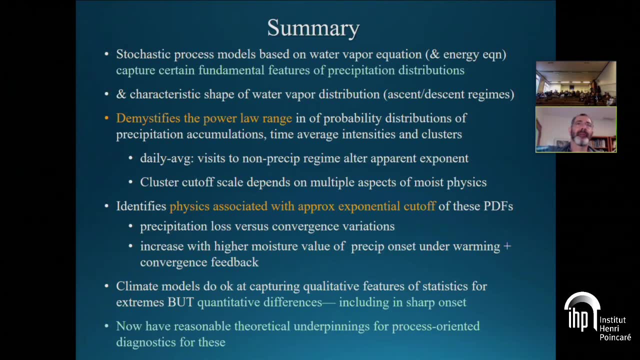 roughly what i said, which is about five times to a grid spacing. i don't have it. i don't have a question. i don't have it. i don't have a question. i don't have it. i don't have a question, it's just a comment. those are all very. 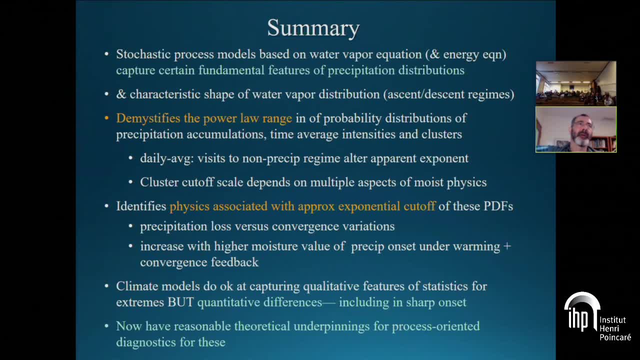 it's just a comment. those are all very. it's just a comment, those are all very good points, good points. good points, um and um. one you know in comparing to um and um, one you know in comparing to um and um, one you know in comparing to observations. of course, one thing you can: 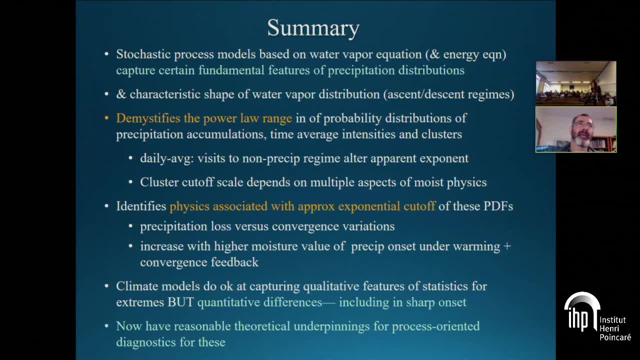 observations, of course. one thing you can- observations, of course one thing you can do is do, is do is statistic. you're interested in what is statistic. you're interested in what is statistic. you're interested in what is the dependence on the, the dependence on the, the dependence on the spatial scale, that's one thing, that is. 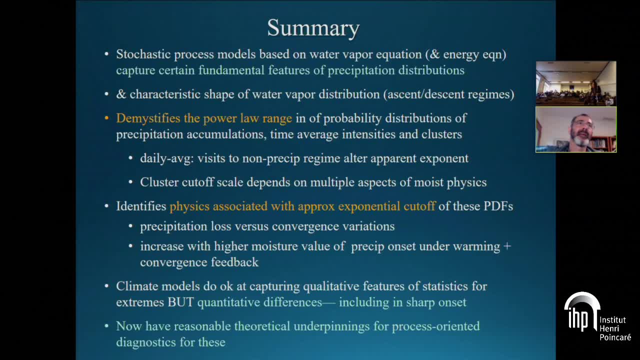 spatial scale, that's one thing. that is spatial scale, that's one thing that is worth, worth, worth what necessarily does, what necessarily does, what necessarily does, but, but, but. one remark from one remark, from one remark, from the results here is that, the results here is that the results here is that, for some aspects of the distributions, 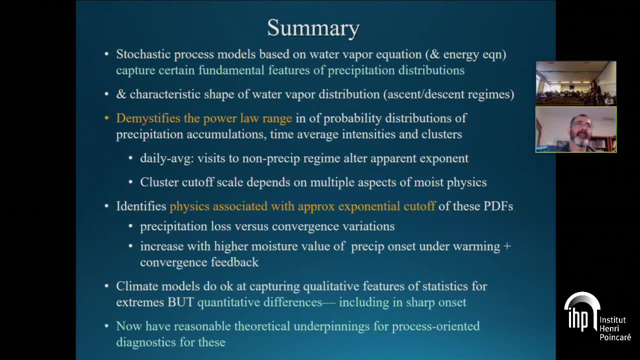 for some aspects of the distributions, for some aspects of the distributions, a very simple stochastic model, a very simple stochastic model, a very simple stochastic model is. is is giving you explanations of the observed, giving you explanations of the observed, giving you explanations of the observed form of the distribution. 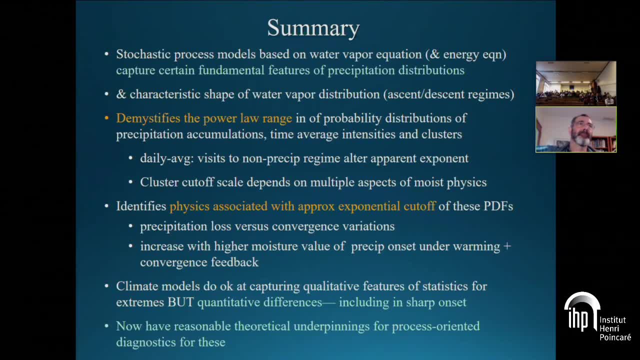 form of the distribution. form of the distribution, including out to quite high. you know precipitation intensities, you know precipitation intensities, you know precipitation intensities, and that means that there's something, and that means that there's something, and that means that there's something fundamentally simple about what's going. 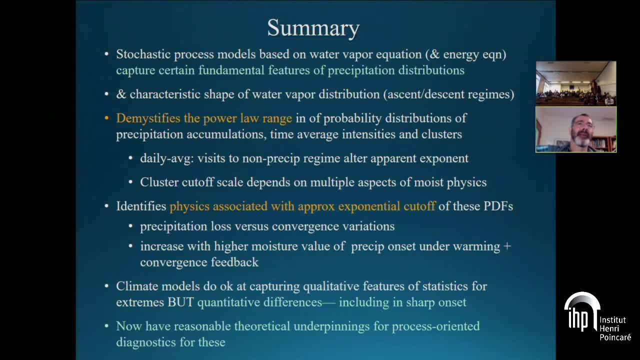 fundamentally simple about what's going, fundamentally simple about what's going on on. on, wherever we have simplicity, we should. wherever we have simplicity, we should. wherever we have simplicity, we should exploit that, because precipitation exploit that, because precipitation exploit that, because precipitation is, as you mentioned, a complex process. 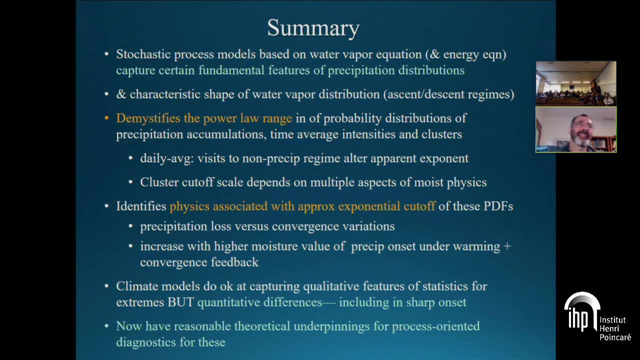 is, as you mentioned, a complex process, is, as you mentioned, a complex process. so, knowing that there are some simple, so, knowing that there are some simple, so, knowing that there are some simple underlying considerations that are underlying considerations that are underlying considerations that are governing, governing, governing, uh, essentially all the um percentiles of 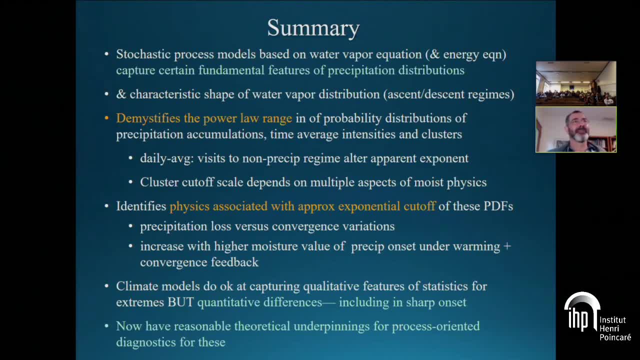 uh, essentially all the um percentiles of, uh, essentially all the um percentiles of the distribution, the distribution, the distribution, except perhaps the very unusual event, except perhaps the very unusual event, except perhaps the very unusual event. um, uh, is is highly worthwhile. um, uh, is is highly worthwhile. 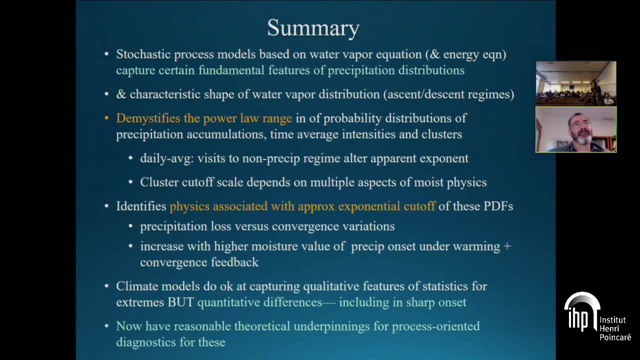 um, uh, is is highly worthwhile and in some sense, as you add resolution, and in some sense, as you add resolution, and in some sense, as you add resolution, of the models, of the models, of the models, this would say: you're just you're, this would say you're just you're. 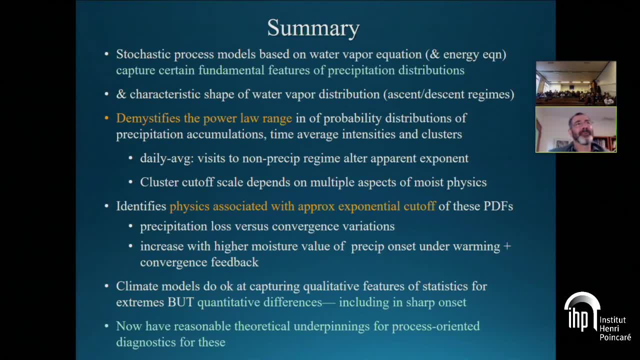 this would say: you're just. you're essentially having an expensive, essentially having an expensive, essentially having an expensive noisemaker from the point of view of noisemaker, from the point of view of noisemaker from the point of view of some of the features of the. 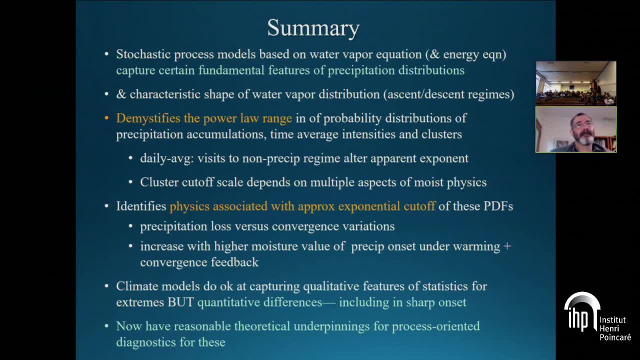 some of the features of the, some of the features of the precipitation distribution: precipitation distribution. precipitation distribution. right right, right. thank you, david um. we, thank you, david um, we thank you, david um. we, we're a little bit pushed by the time. so we're a little bit pushed by the time, so